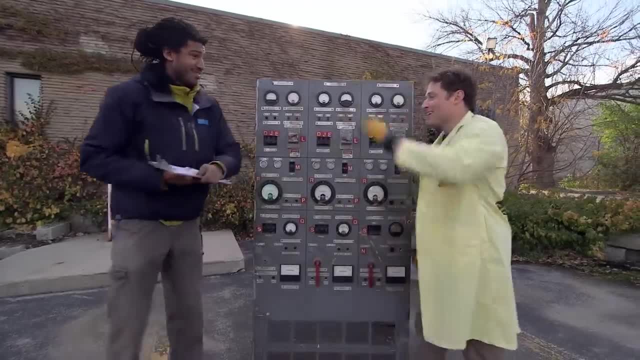 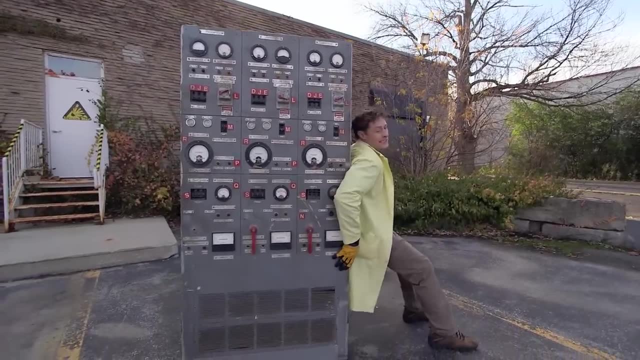 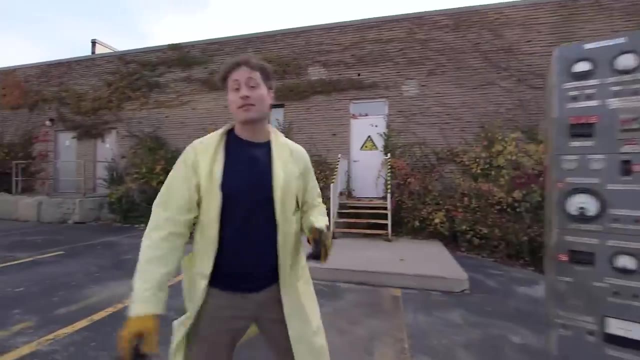 Thanks very much, No problem, I appreciate it, Enjoy. Thank you. Well, my very own particle impulse controller. Okay, That's as heavy as I thought I was going to be. All right, Science Maximites. This episode of Science Max Experiments at Large- is going to be a little different. 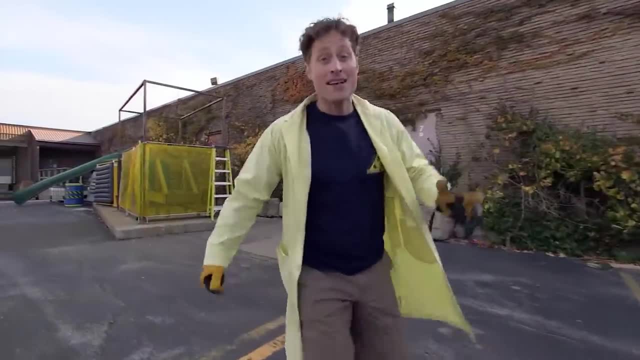 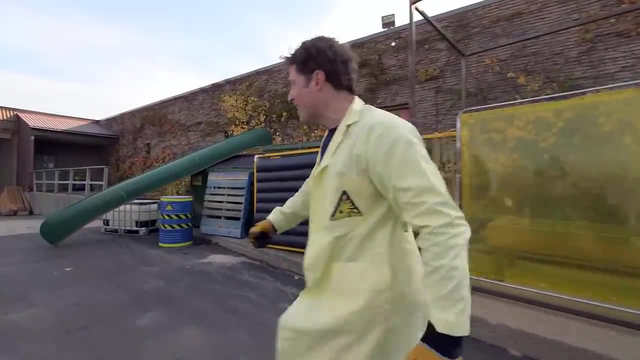 Because today I'm not going to have an expert come and help me, Because I'm going to move that giant heavy particle impulse controller all the way across the parking lot, All the way up that loading ramp by myself, with nobody's help. 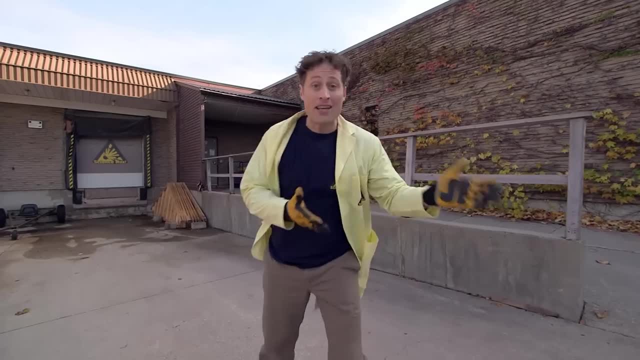 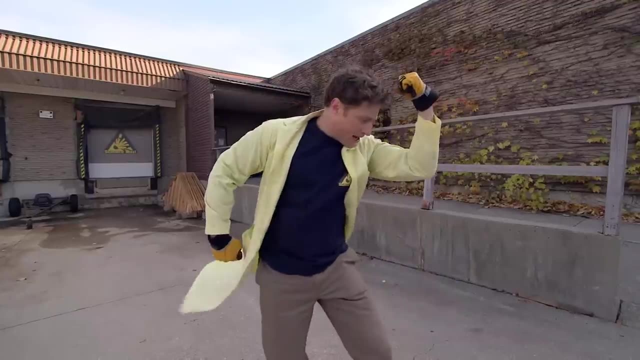 How am I going to move a giant heavy machine all that way if I can barely even budget? Well, I'm going to give myself super powers, super strength, with the power of simple machines, And the first machine we're going to start with is the lever, which I guess I should. 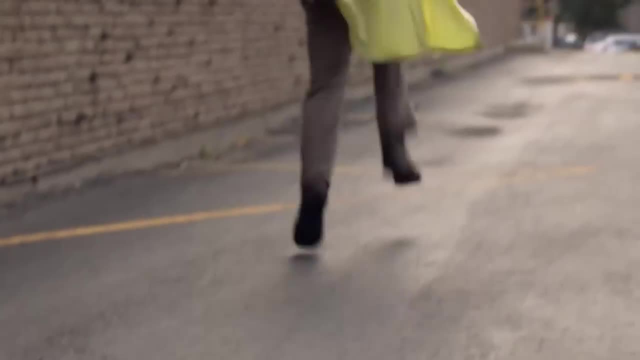 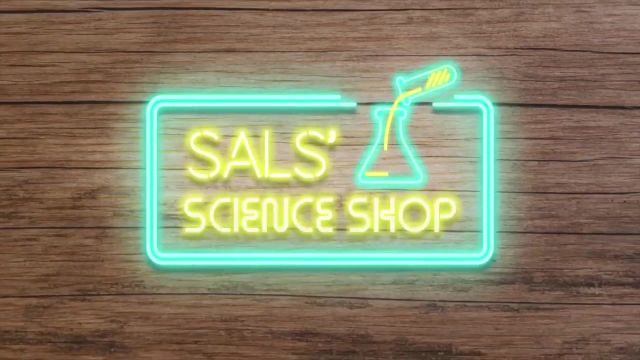 go back to the lab to tell you about. All right, Sal, I'll see you next time. Oh hey, How are you doing? Let me guess You've got some work to do when you need it done, easy, right. 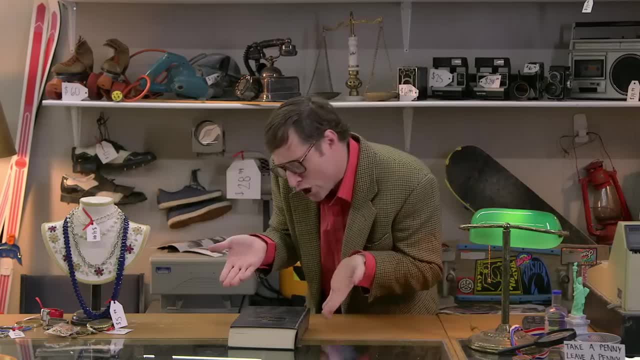 I mean, look at this book. I mean you could pick it up. But what Are you going to be some sort of book-picker-upper person now? Is that all you're going to do? Is that going to be your life, just picking up books left, right and center? 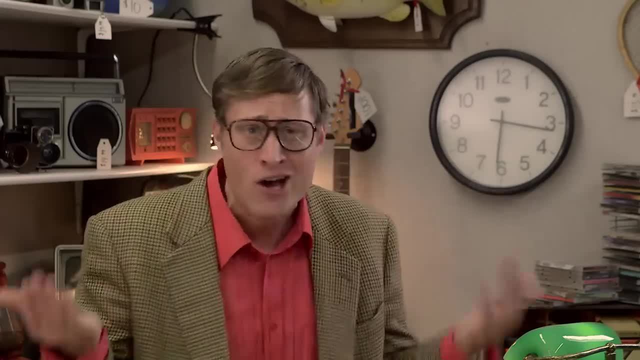 No, You're smarter than that. You know what you need: A lever Like this. Now, I know what you're thinking. I know You're thinking: hey, this is just a plank. You're right, That's because you're smart. 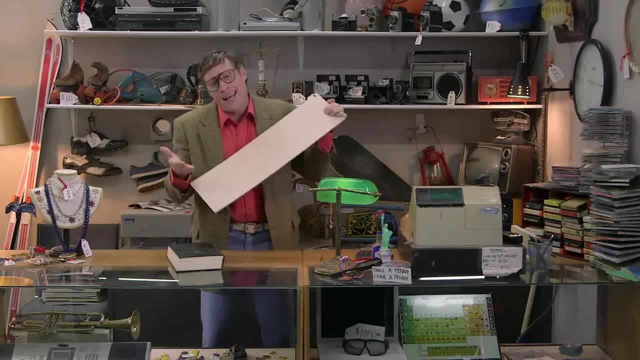 You know what you need: A lever. Now, I know what you're thinking. I know You're thinking: hey, this is just a plank. You're right, That's because you're smart. A plank can be a lever. 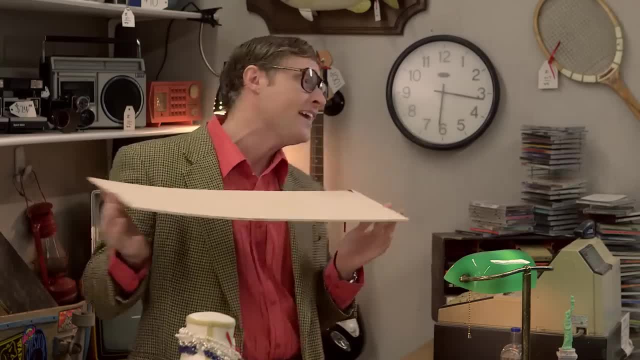 All you need is two sides and a place for it to pivot- A fulcrum. It can be anything. Look at this, Bam. Now it's pivoting. I put the book on this side and then I push down on that side. 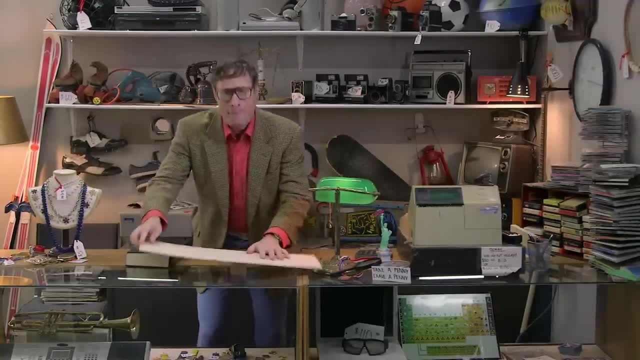 I'm doing work easy. Hey, look at me doing this work over here. If I want to do more work, I could move the fulcrum a little bit further over. Now it's pivoting. I put the book on this side and then I push down on that side. 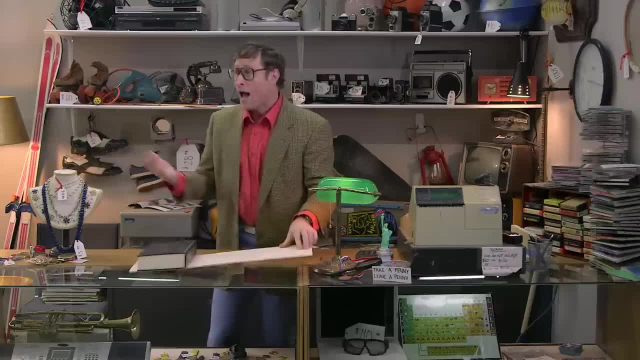 I'm doing work easy. Hey, look at me doing this work over here. If I want to do more work, I could move the fulcrum a little bit further over. Now. I do lots of work, but I lift the book a lot further. 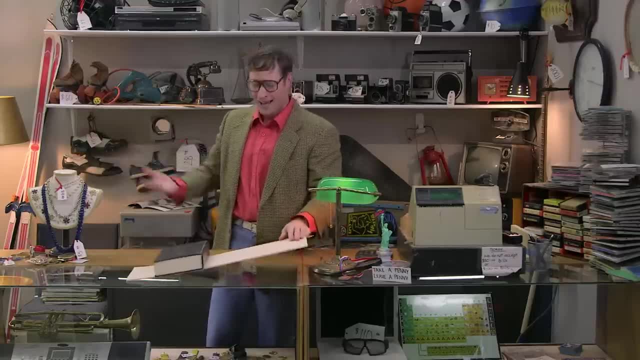 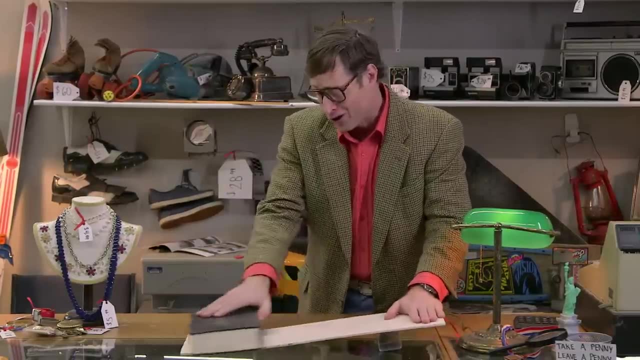 Look at that: Whoa, What, Whoa, Yeah, Huh. What do you say? What do you say? Huh, Huh. You don't like this lever, Don't worry, Hold on, I got another one for you here. 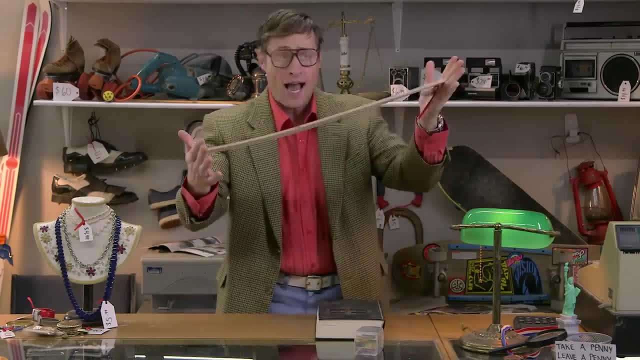 Hey, take this stick. All you need is two ends and a place for it to pivot, Like this Bam. Now it's a lever. All you need is two ends and a place for it to pivot, Like this Bam. 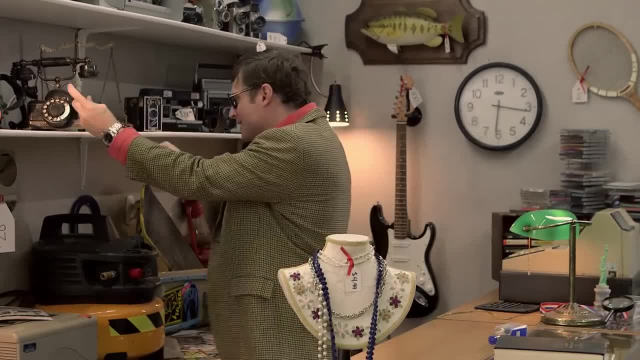 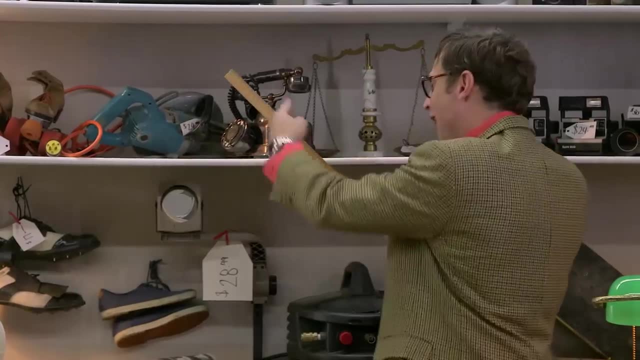 Now it's pivoting. All you need is two ends and a place for it to pivot, Like this Bam. Now it's pivoting. Two ends and a place for it to pivot Like this Boom. All you need is two ends and a place for it to pivot. 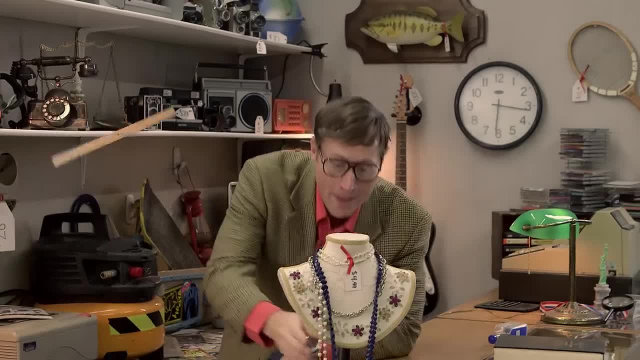 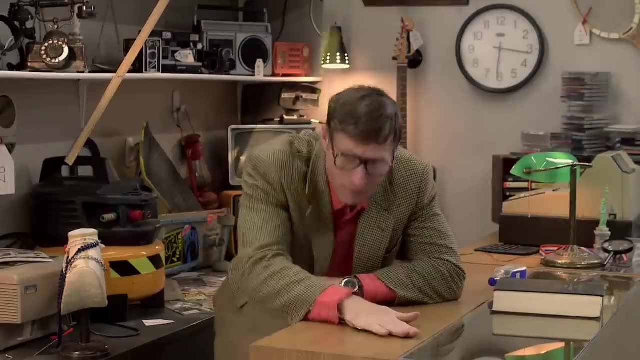 Bam. All you need is two ends and a place for it to pivot Like this Bam. Now it's a lever. This side goes down, That side goes up, Down, Up, It's a lever, It's a lever. 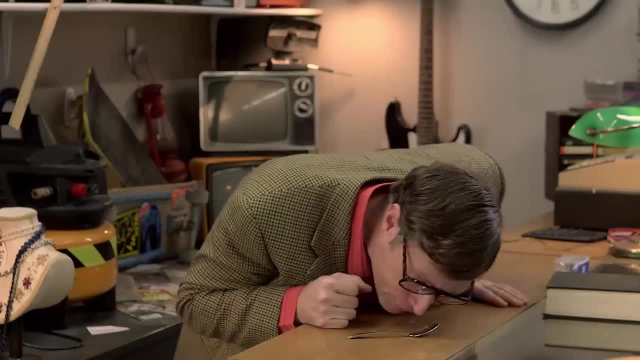 You want to make a catapult, use a spoon. The place where the spoon pivots is the fulcrum, And now it's a lever. It's a lever, It's a lever. Look at this lamp. Now it's a lever. 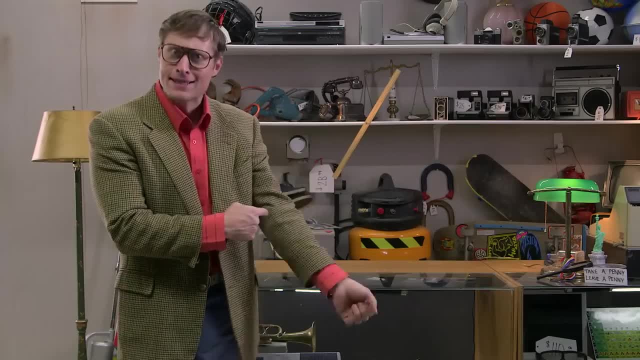 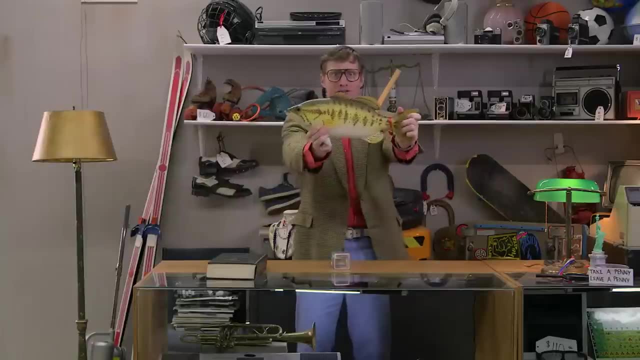 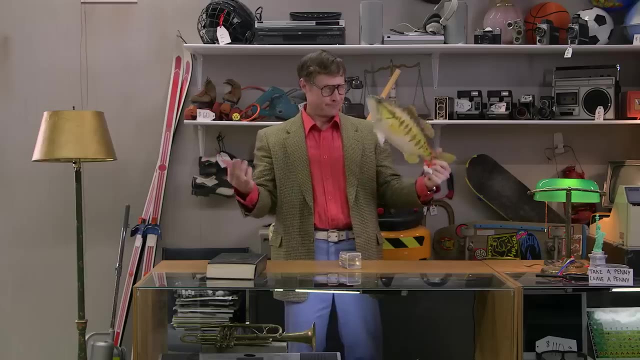 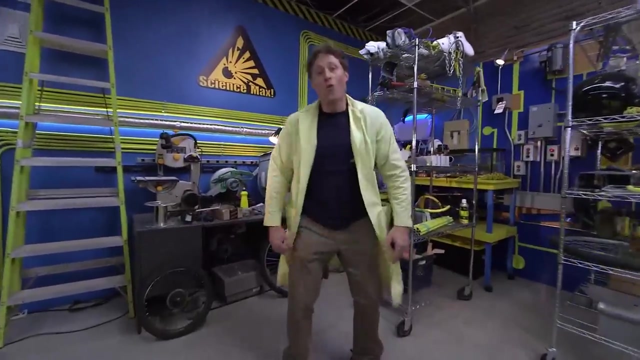 Scissors. Two levers. Your forearm, It's a lever. Two ends the fulcrum where it pivots. Yeah, the fulcrum can be at one end. Crazy, This fish. you guessed it. now it's a lever. And now you know your levers. Okay, where were we? Oh, yeah, levers. 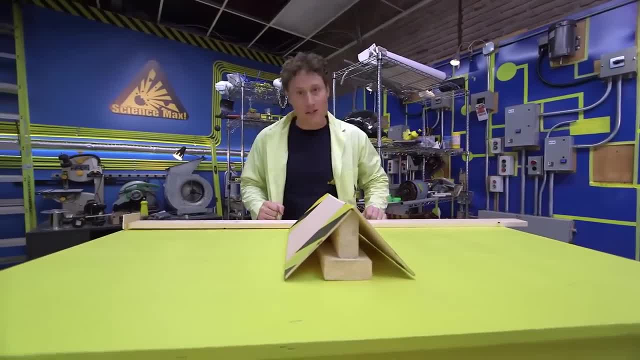 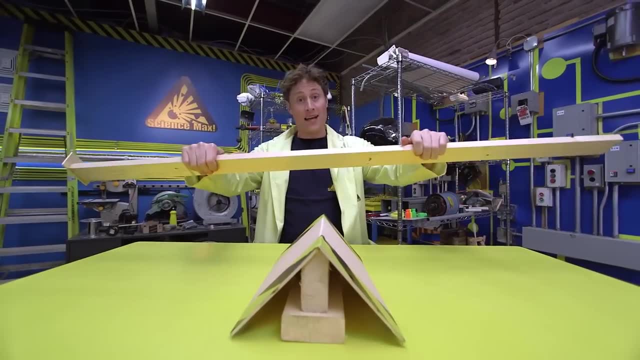 So you can use levers to become much stronger or at least lift something you couldn't normally lift. Levers are simple machines and they work like this. Levers are just a long rod or a stick or pole or a piece of wood, like I've got here, and something for them to pivot. 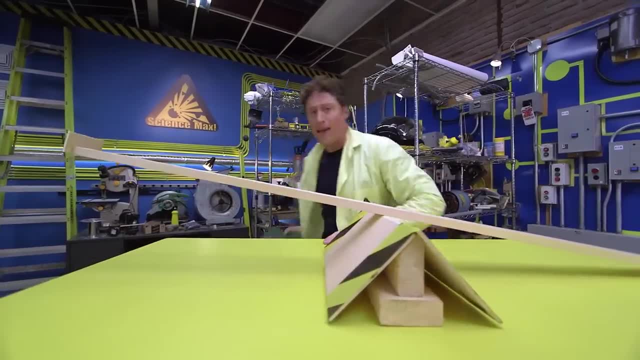 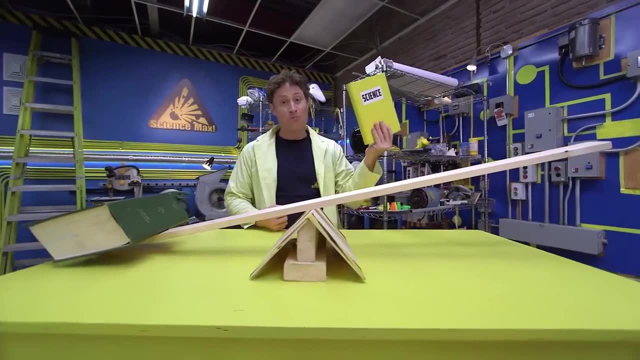 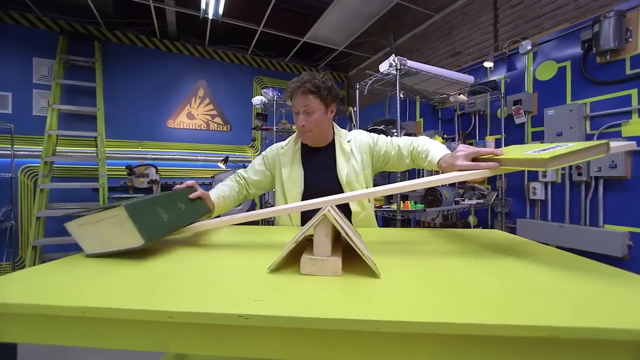 on a fulcrum. Now, let's say you have something heavy like this book, Sure, I can lift it. but what if I told you I can lift this heavy book with this book? Now, if the fulcrum is in the middle like a seesaw, you can tell that book is much heavier than the other book. 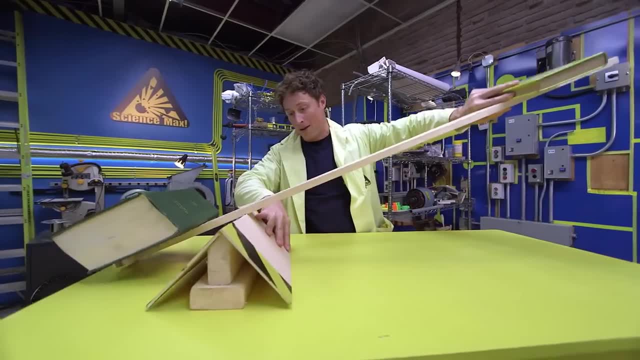 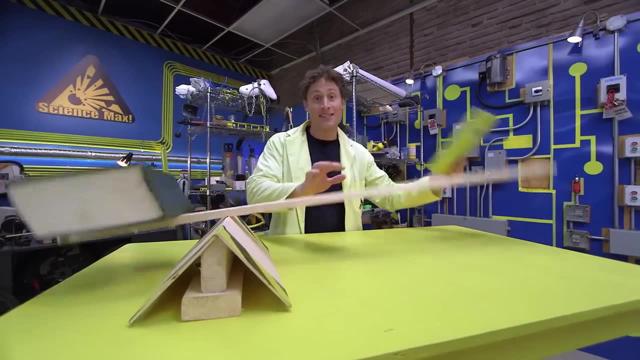 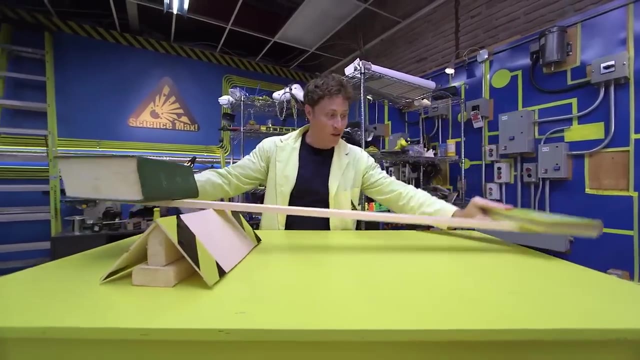 But watch what happens when I move the fulcrum. Huh, It's like magic. but it's not magic, it's science. It's because the small weight is moving a long distance and the heavy weight is moving a short distance. Small weight: 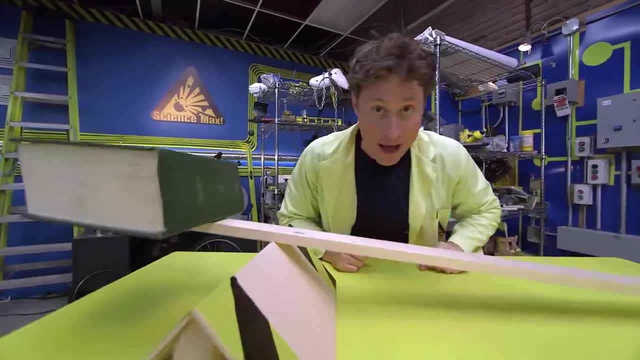 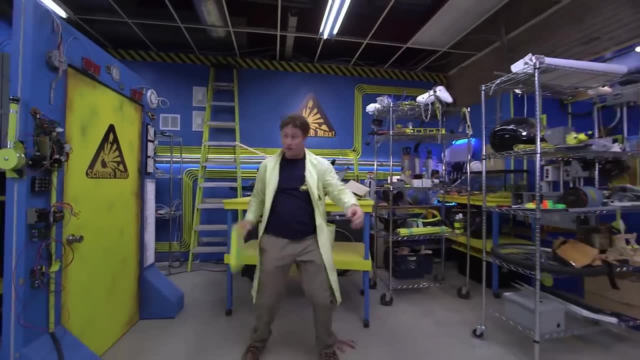 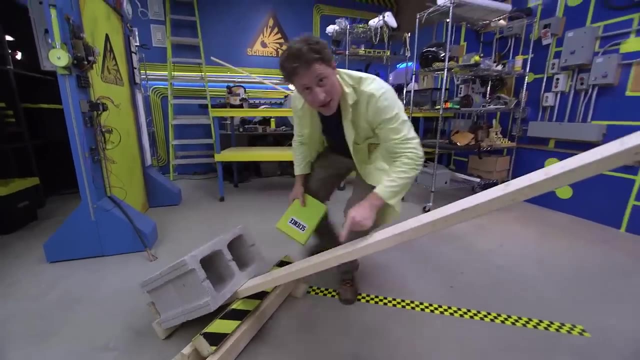 long distance. heavy weight, short distance. So everything balances out. But here's where it gets interesting: The longer your lever, the more weight you can lift. These are the two heavy cinder blocks. There's the fulcrum and here is a very long lever with which. 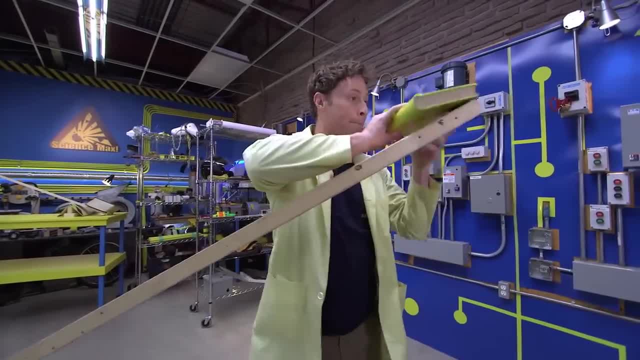 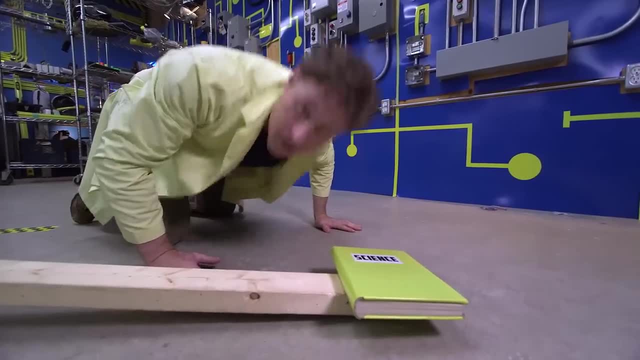 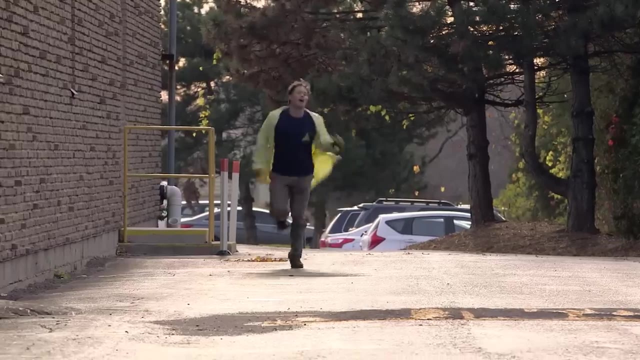 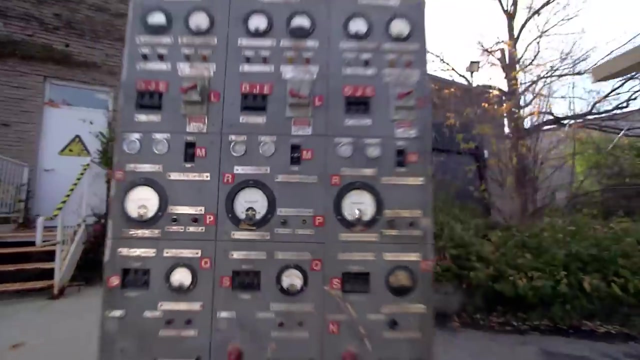 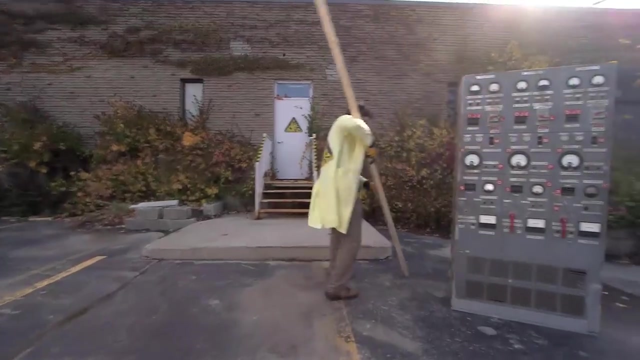 I am going to lift those cinder blocks with this book. Ha ha, And there you have it. Levers. Now back to the particle impulse controller. Oh right, What What? Ha ha, ha, ha, ha. Lever, Here we go, I got my giant lever. The bigger the lever is, the 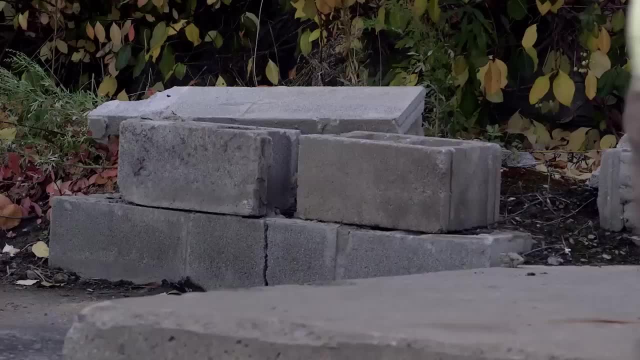 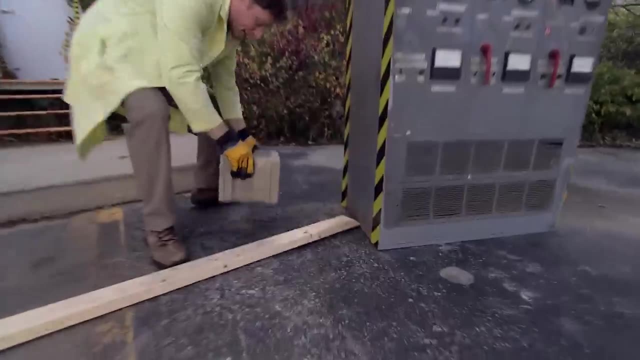 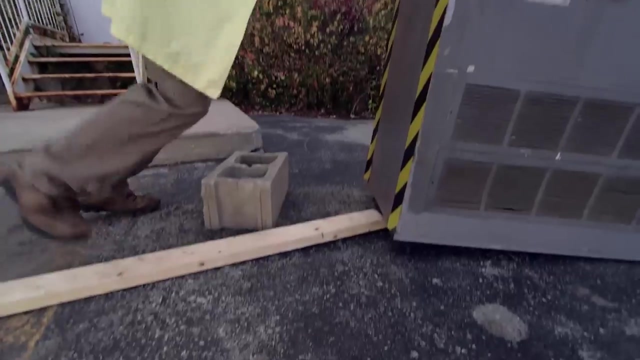 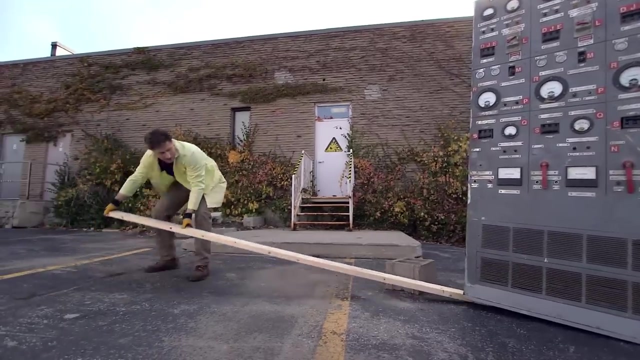 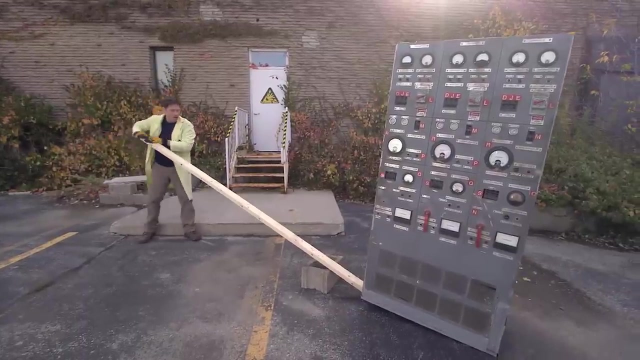 easier it is to do the work. I need a fulcrum. Oh, Just about anything will do for a fulcrum And put that there Now. the hardest part is getting it on the lever. Okay, Okay, Okay, All right, Hardest part is over. Get the lever up on the fulcrum And oh, ho, ho ho. Look at 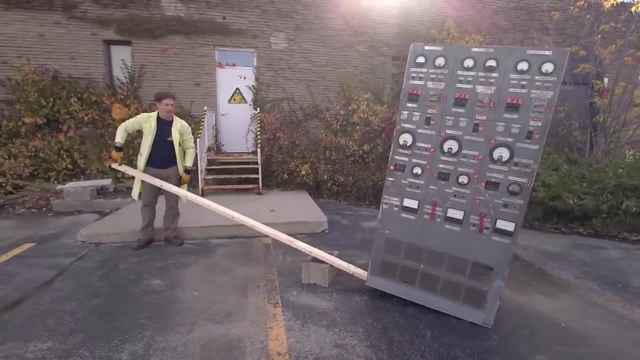 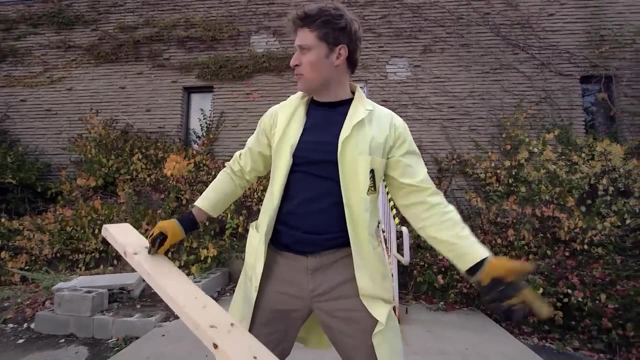 this, No problem. One finger lifting. It suddenly became very easy for me to move this. I guess I need to do more than just lift it, though, huh, Because I have to move it all the way. Oh, Rollers, Come on Back to the lab. 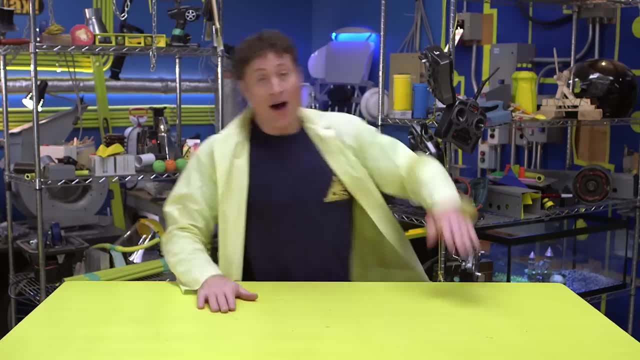 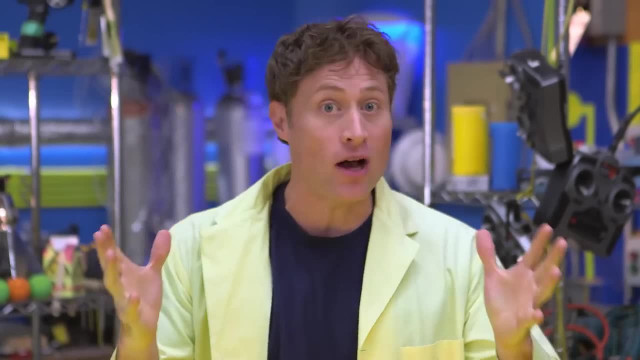 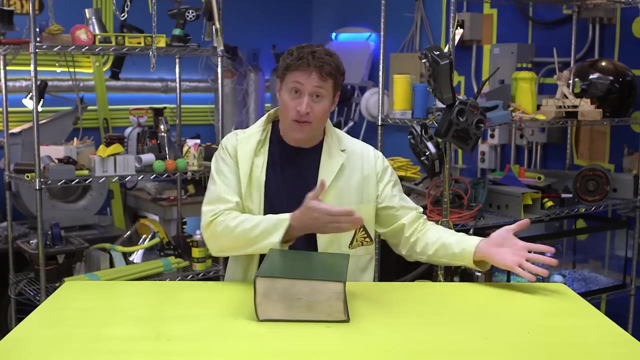 Okay, Rollers. Rollers are like wheels, except they're not attached to anything. In ancient times, they used to move giant, heavy blocks of stone using rollers. We can demonstrate using a book. Now get a book, put it on a table and try to move it across the table. 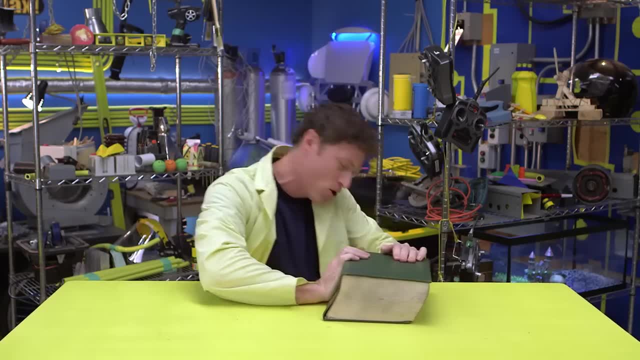 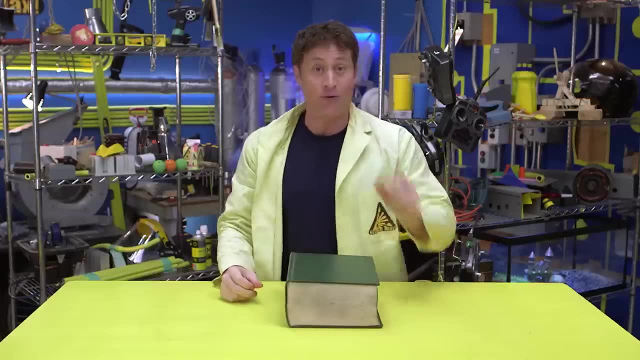 You'll see that it's very difficult. I can't move this book across the table. I can't. Okay, It's not really that hard, But still it takes effort. But if we get some rollers, I like to use pencil crayons and not pencils, And here's why. Take a closer look, You see. 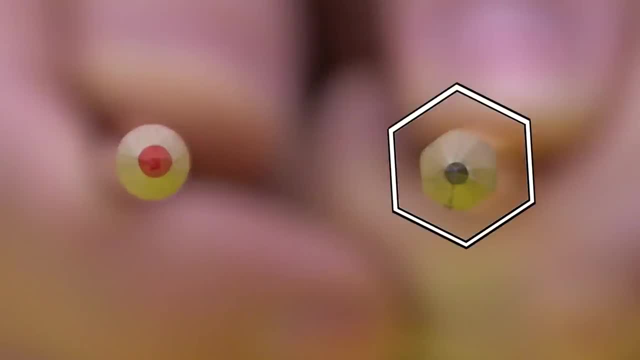 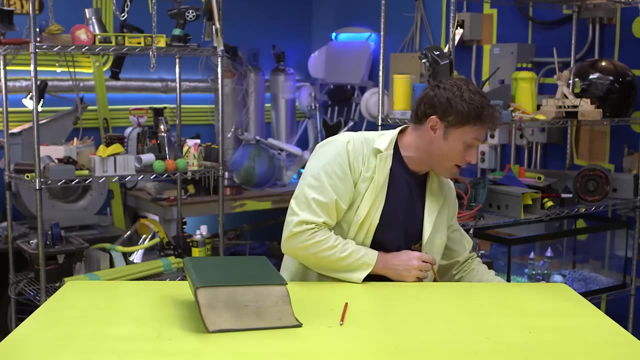 pencils aren't round, They're hexagonal, They have six sides, Whereas pencil crayons are round And, of course, if you want something to roll, you want something round. So get a bunch of pencil crayons and put them on the table And put the book on the pencil. 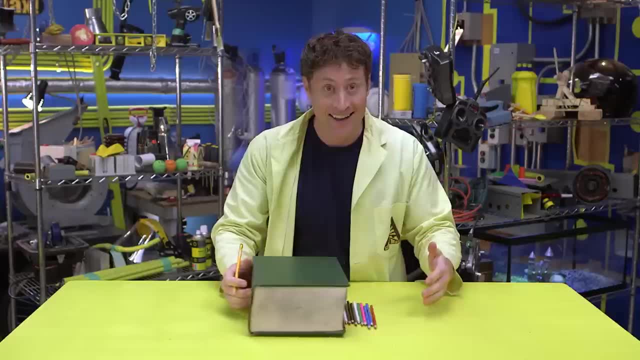 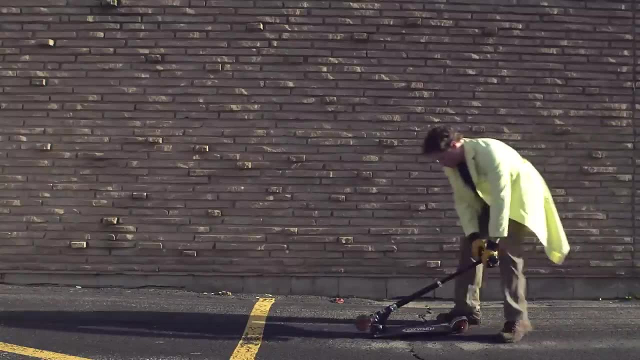 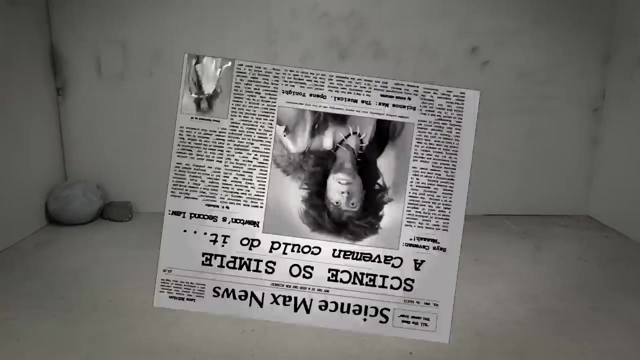 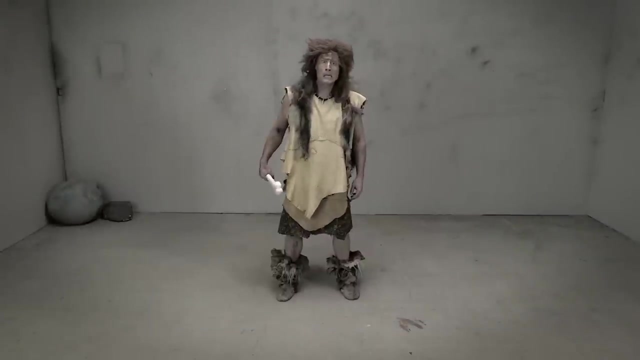 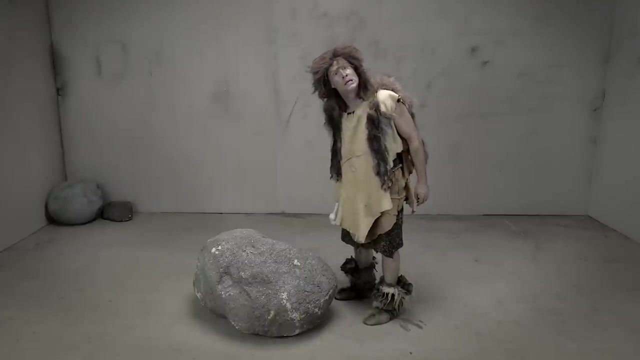 crayons And you'll see that suddenly moving it is a lot easier. All right, That's rollers. Back I go. Now it's time for science. so simple a caveman could do it. This is a caveman, This is a rock. It is a well-known scientific fact that if this caveman were to try to move, 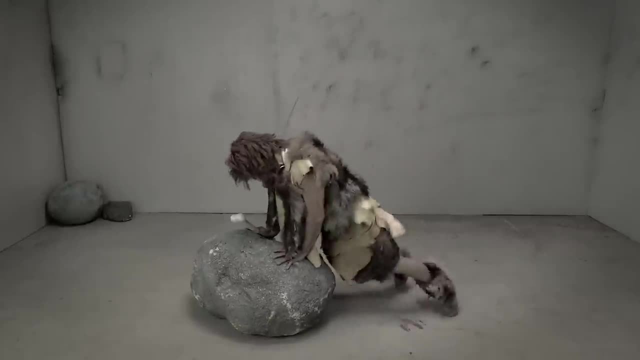 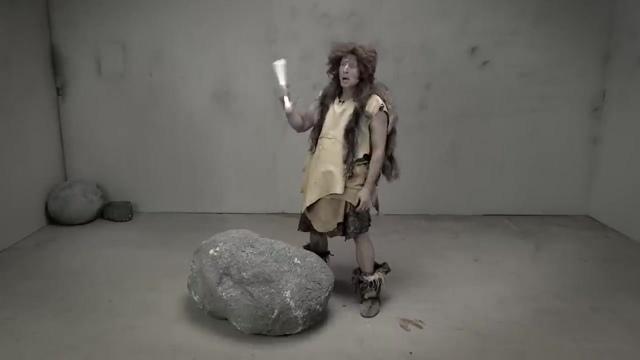 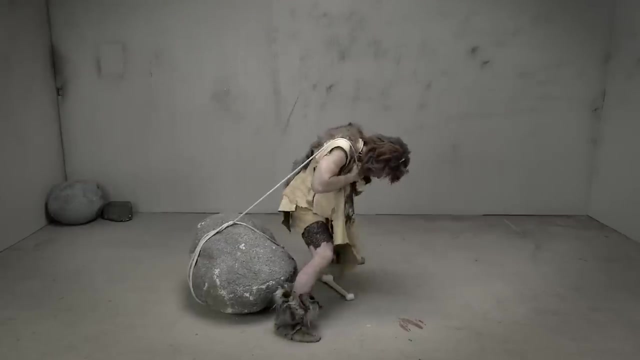 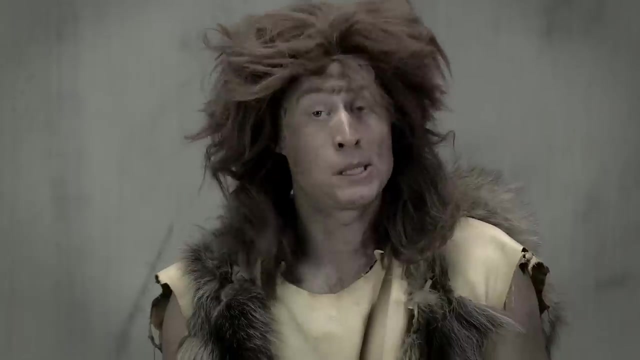 that rock. he would not know how to do it easily, Poor caveman. But in ancient times people learned how to move heavy rocks using ropes and rollers. Oh, Rollers, Yes, Rollers, Rollers, Rollers, Rollers. 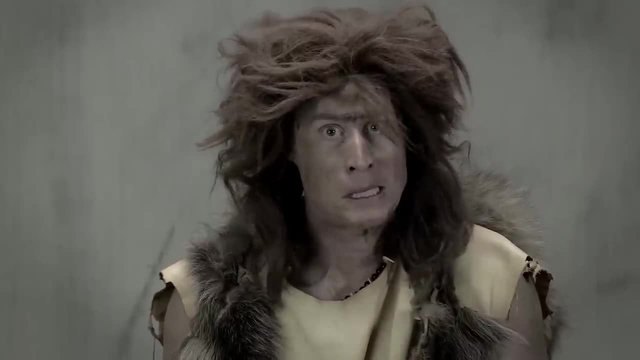 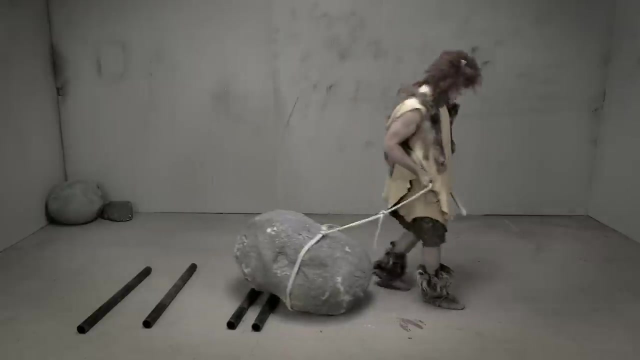 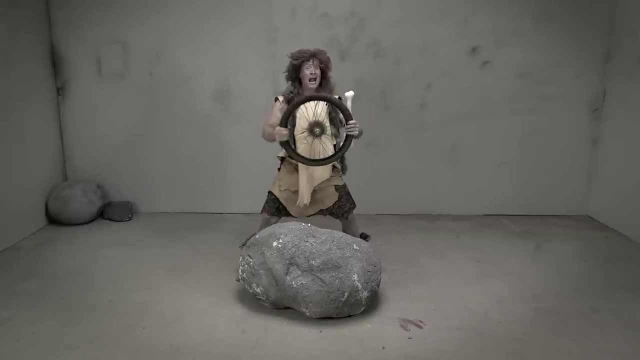 Close enough. Rollers make it much easier to move Rollers, Rollers, Rollers, Rollers, Rollers, Rollers. But they aren't perfect, So the wheel was invented. The wheel is a simple machine and one of mankind's greatest inventions. 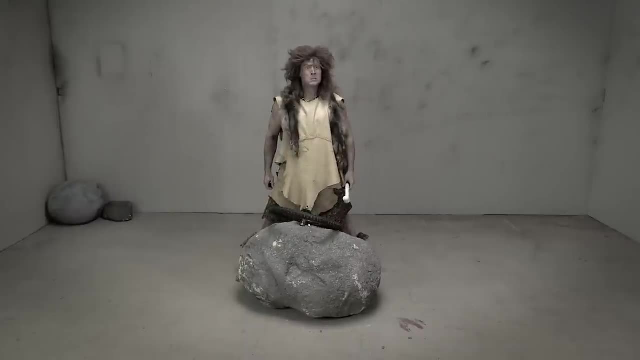 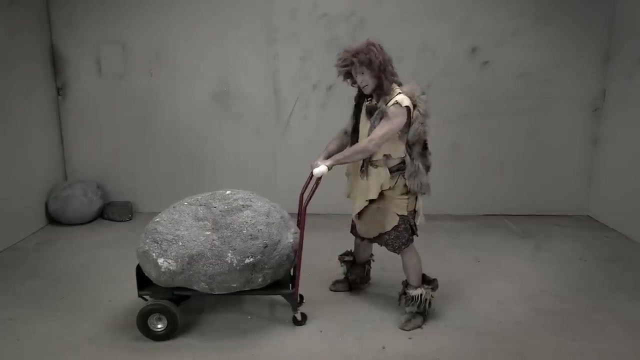 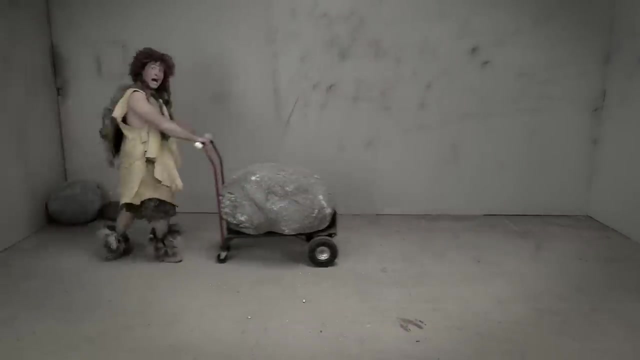 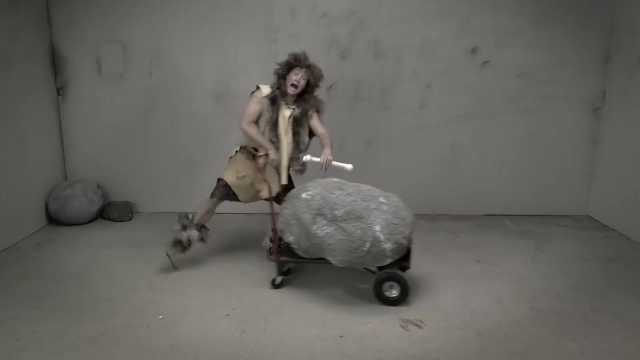 No, that's not how it works. No Wheels go on axles which go under a platform. Now you have something to place that heavy rock on to move it around. but all these great inventions came after the time of the caveman. caveman had to do everything the hard way. join us next time for more. 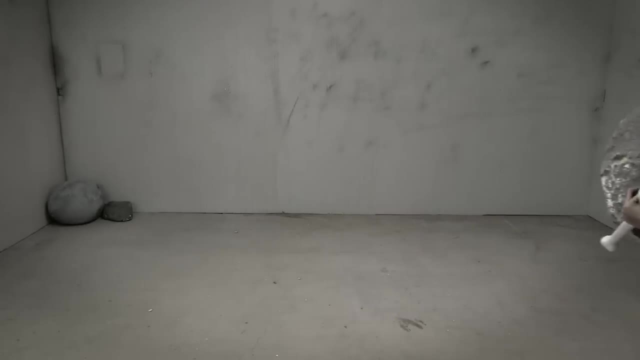 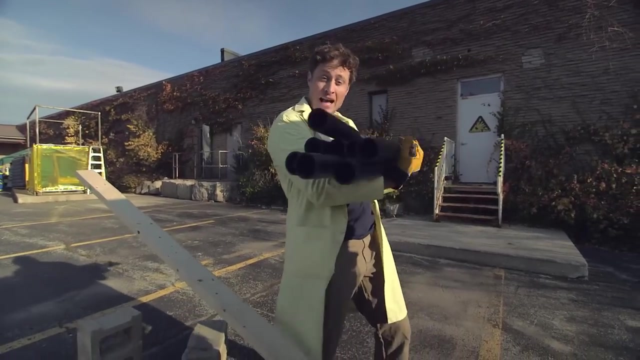 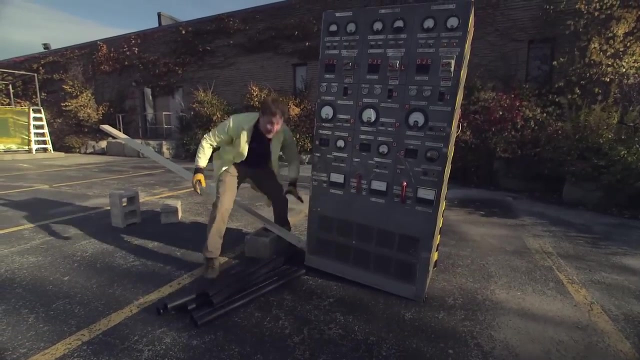 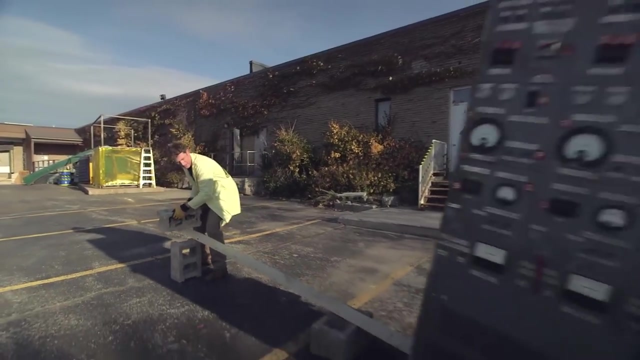 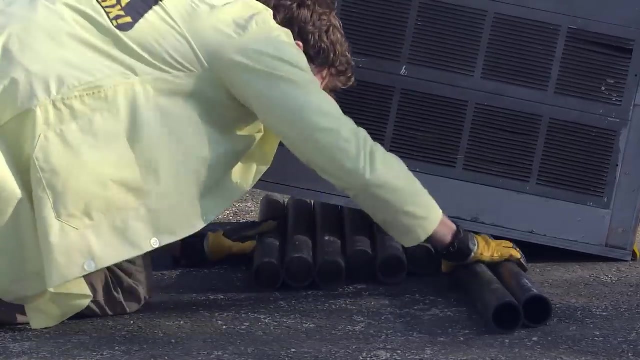 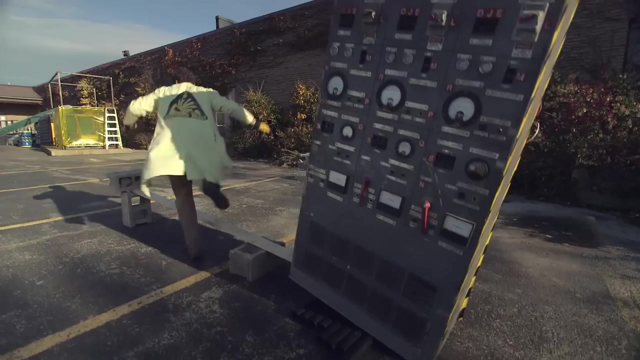 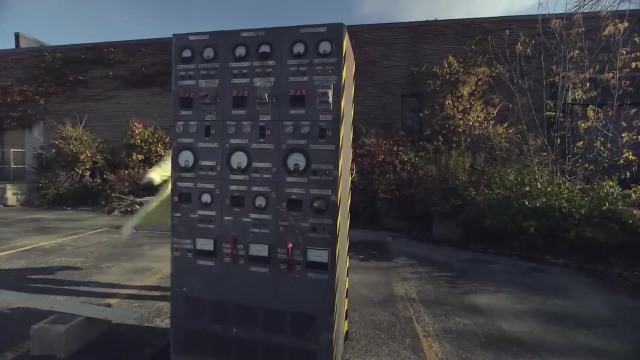 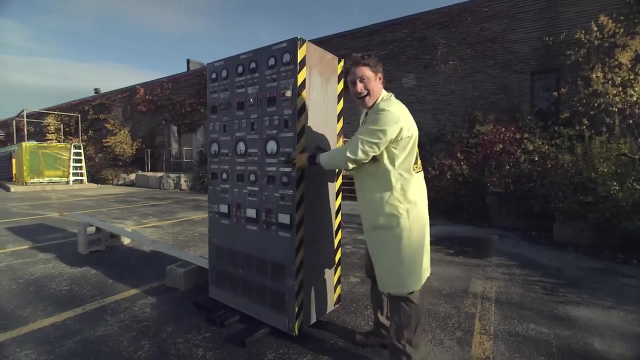 science. okay, I've got rollers. they're just plastic pipes, but they'll work perfectly. I put them, and now to lift up the machine, perfect. and so the rollers go underneath like that. and then, whoa, whoa, careful, uh-huh, look at that, no problem, wait, I gotta get rid of this. 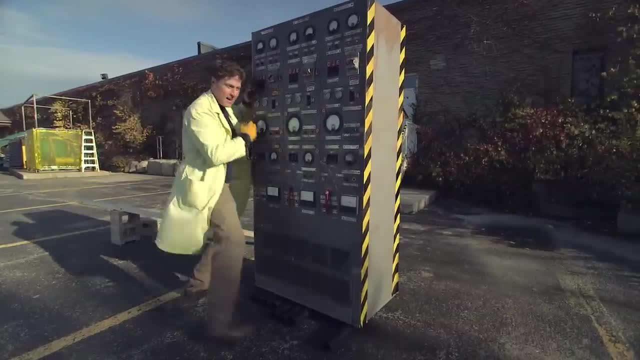 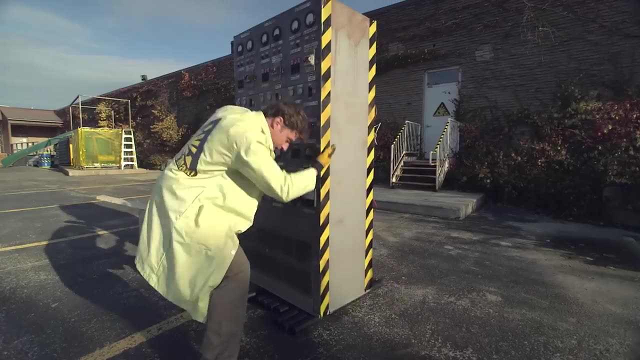 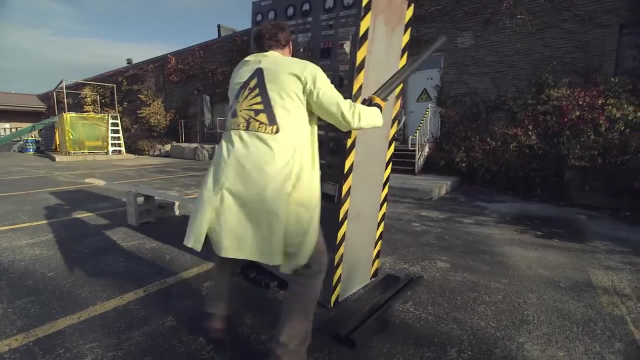 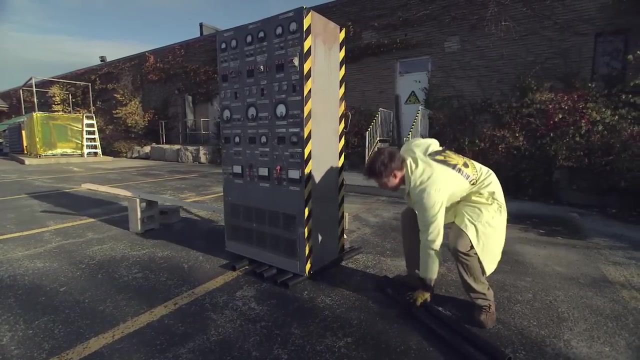 get it. okay, movie. now. the trick with rollers is you have to keep taking them out of the back and putting them in the front. but whoa, whoa, whoa, it's stop, rollers, stop. oh no, oh, no, okay, okay, whoa, rollers. easy, there we go. okay in the front, roll it forward. 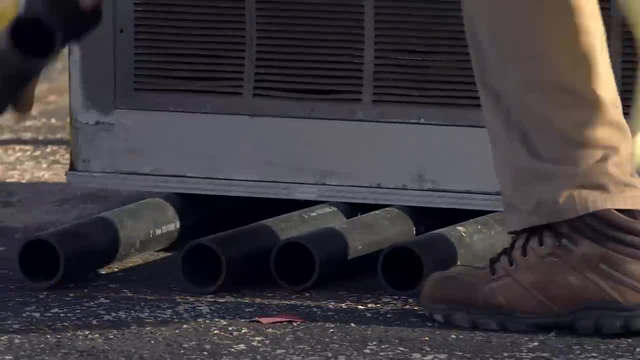 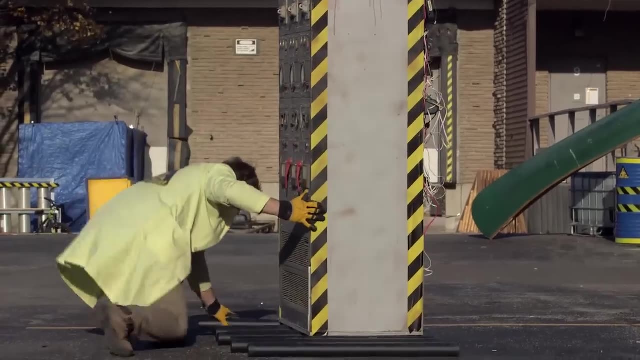 now I know what- You're thinking. this seems like a lot of work, And it's true. moving the rollers back and forth and back and forth does take some time. But did you know? this was how the pyramids were built. It's true. 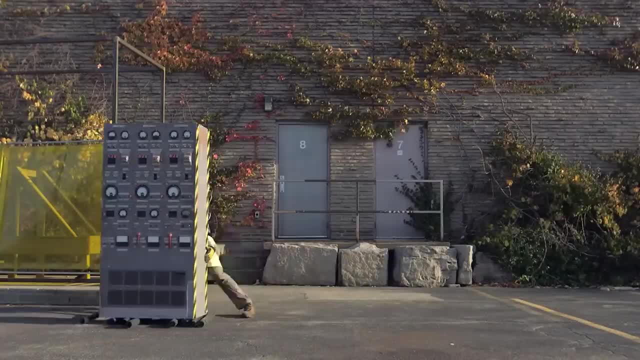 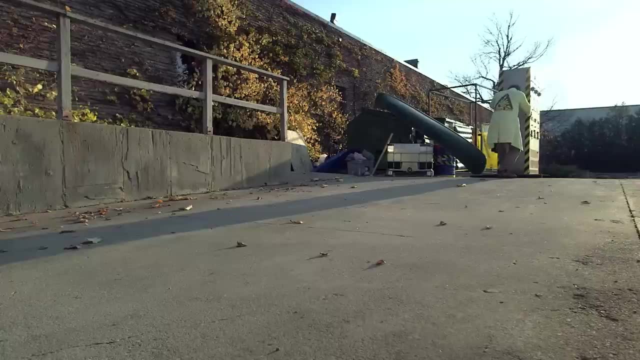 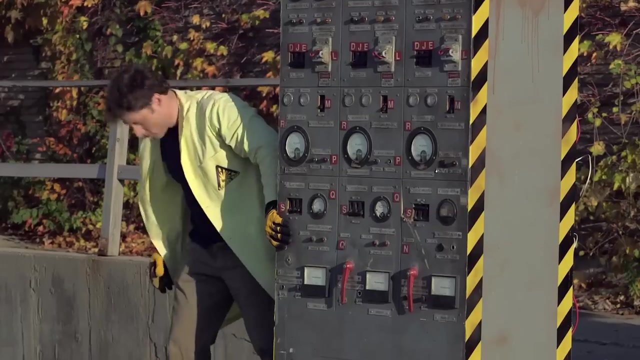 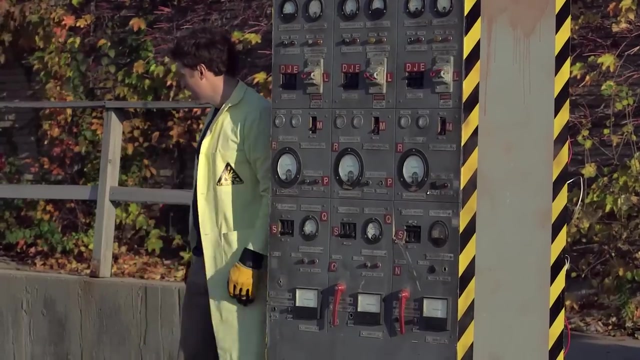 Giant stone blocks were moved on rollers, just like I'm doing here, And, as you can see, what worked for the ancient Egyptians works for me too. Uh-oh, Yeah, there's a hill here. Um, if I go down the hill, 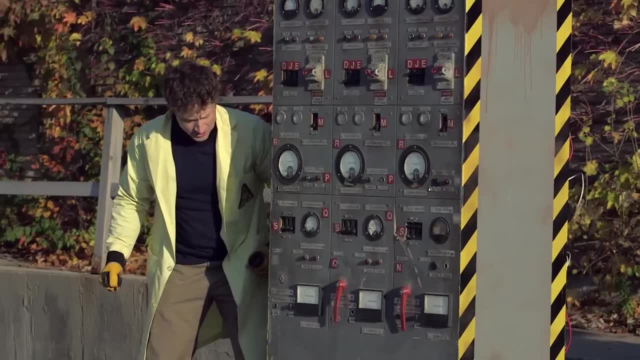 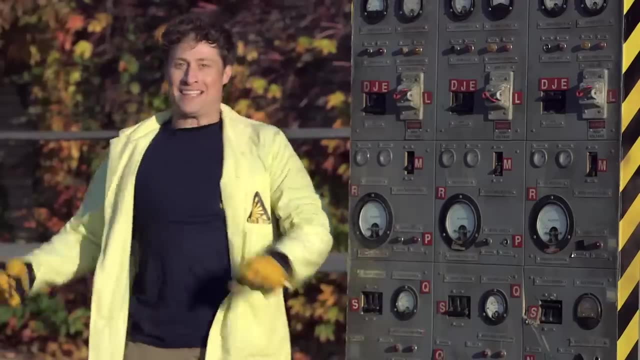 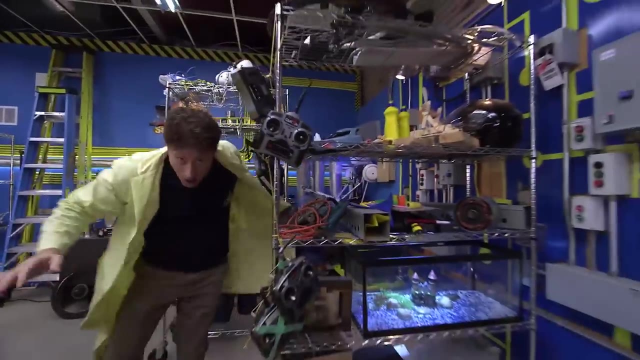 it's gonna start rolling faster than I can do the rollers. I'm gonna need some help. Um uh, Oh, I know, Pulleys, Pulleys, Pulleys, Okay, Pulleys, Pulleys are a great way to change the direction of force. 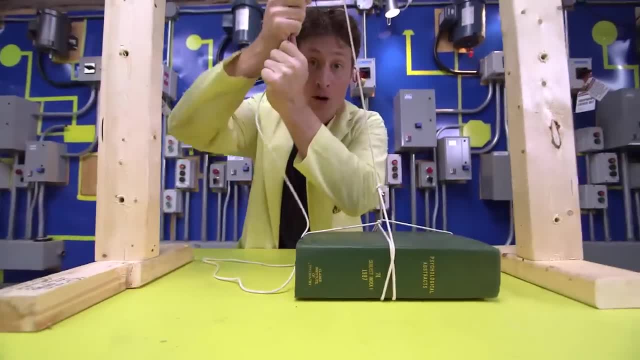 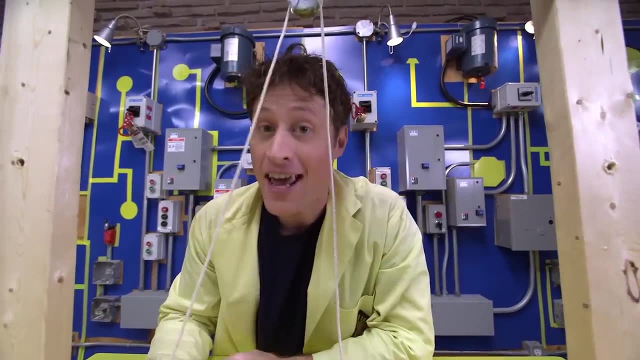 I've got a rope going through this pulley and down to a book. So when I pull the rope down, the book goes up. Changing the direction of force can be very helpful, but pulleys can be helpful in another way. Pulleys can let you lift something. 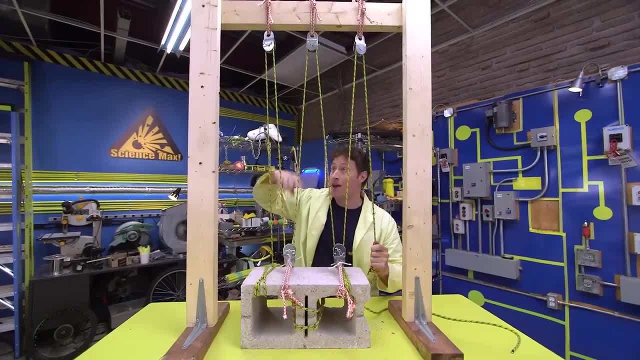 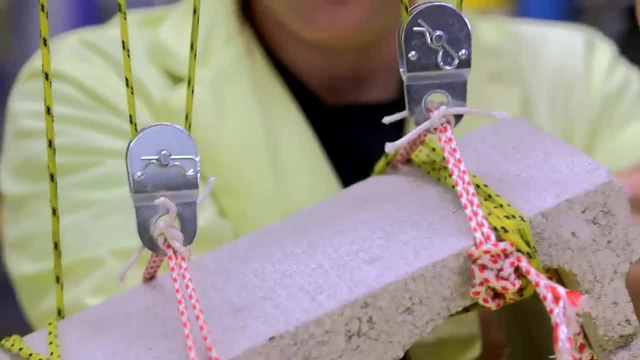 that you couldn't normally lift. Now the rope goes up and down, and up and down, and up and down, And the force I need to lift this cinder block is a lot less than if I was just lifting it by myself, But I've got to pull a lot more rope. 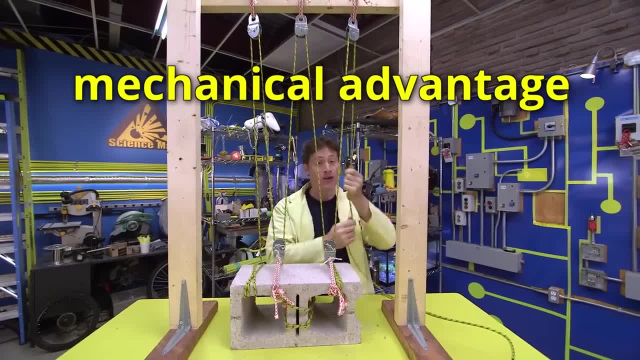 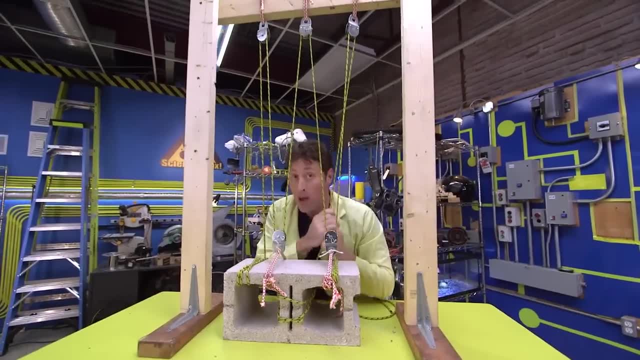 That's called mechanical advantage, Spreading out the force over a longer pull so you can lift a larger weight. If you use more pulleys, it reduces the amount of force. One pulley: same amount, Two pulleys: half the force. 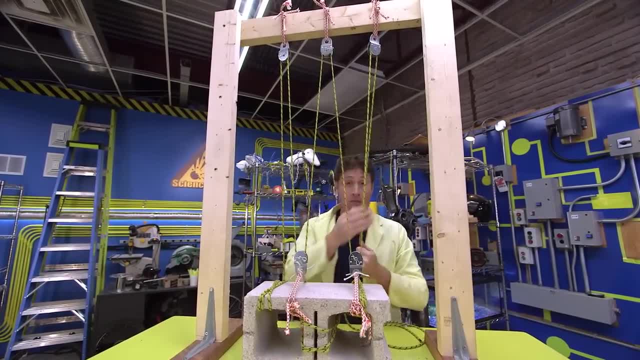 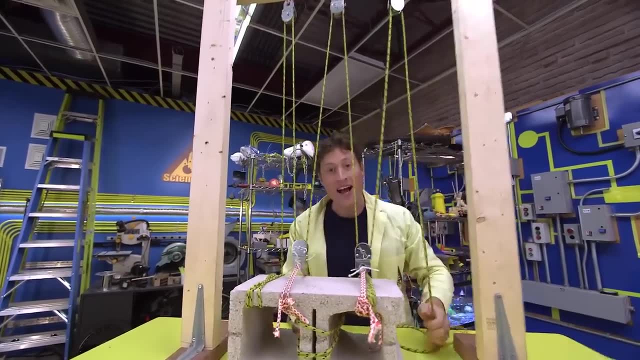 Three pulleys, one third. So I've got five pulleys here, which means I only need one fifth of the force to lift this cinder block. So there you go, pulleys. Now back to the wait a minute, wait a minute. 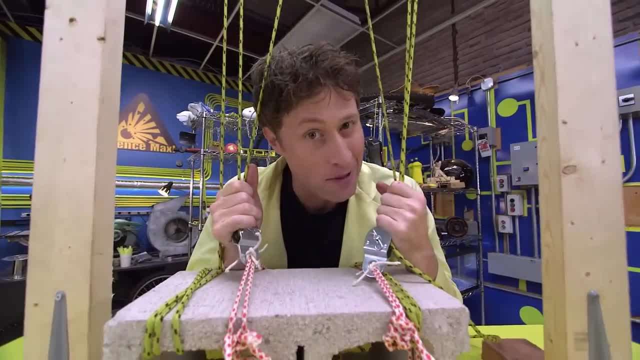 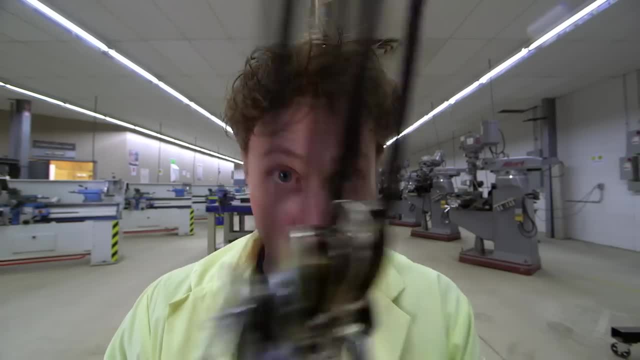 This calls for a mini-max, Mini-max. So how much weight can you lift with pulleys? Well, as much as you want, really. I have four pulleys on the bottom and four pulleys at the top. That means with eight pulleys. 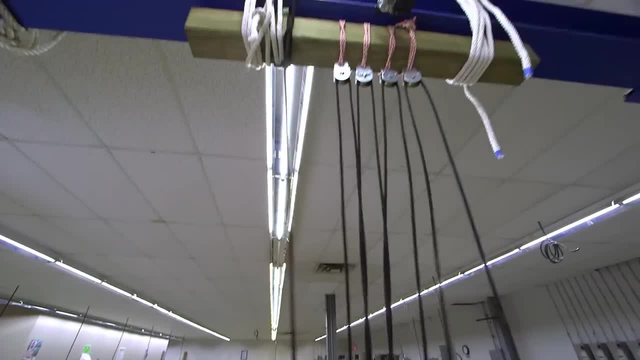 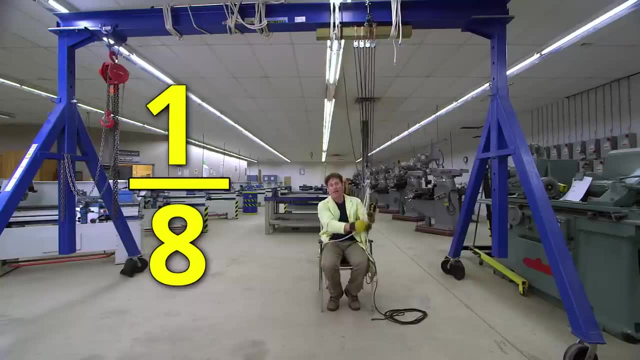 I only have to lift one eighth of my weight plus the weight of the chair I'm sitting in. So I've got four pulleys on the bottom and four pulleys at the top. That means with eight pulleys I only have to lift one eighth of my weight. 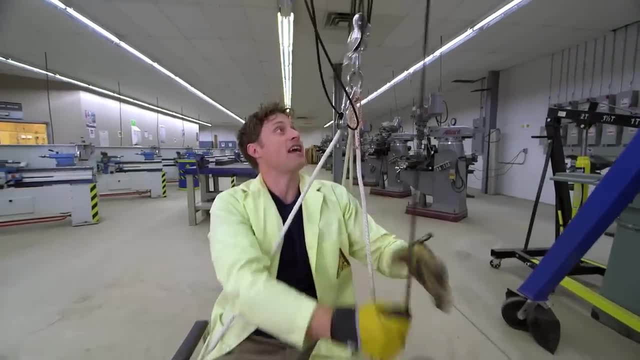 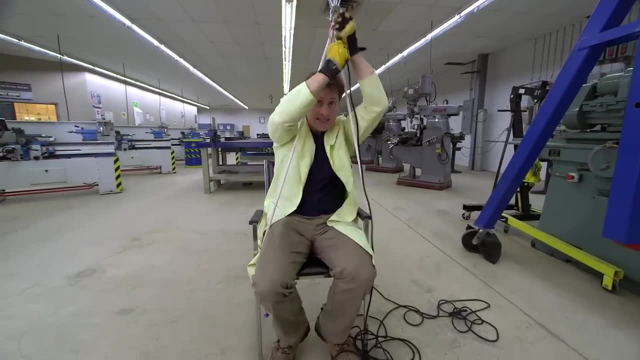 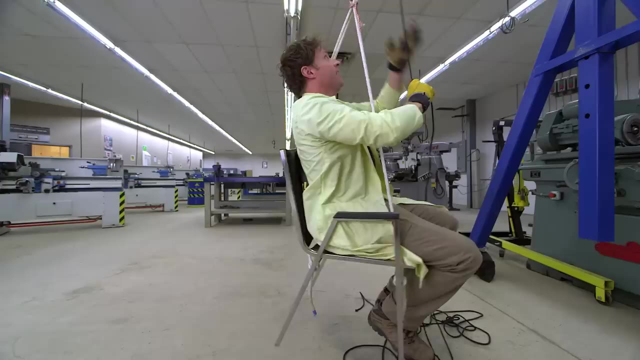 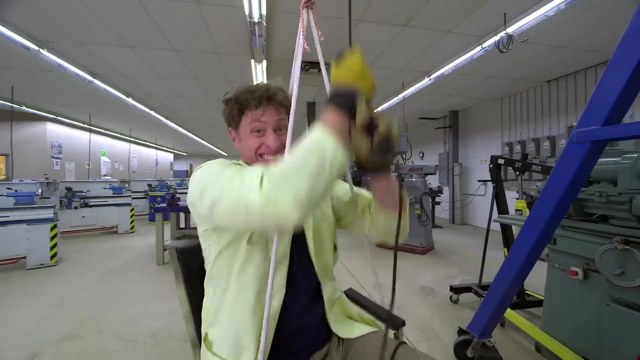 and if I keep pulling, you will see that the chair I'm sitting in is roped to the pulleys. So now we see if I can pull myself up with nothing but pulleys. Look at that, I'm totally lifting myself into the air. 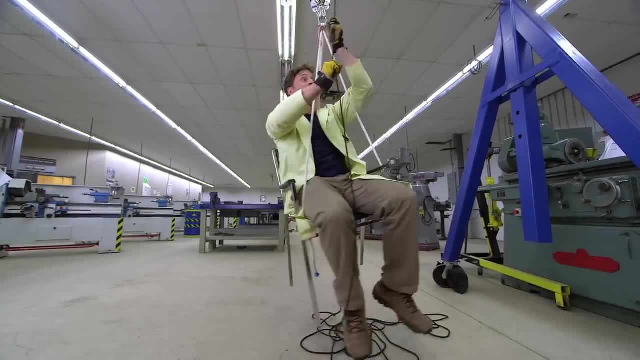 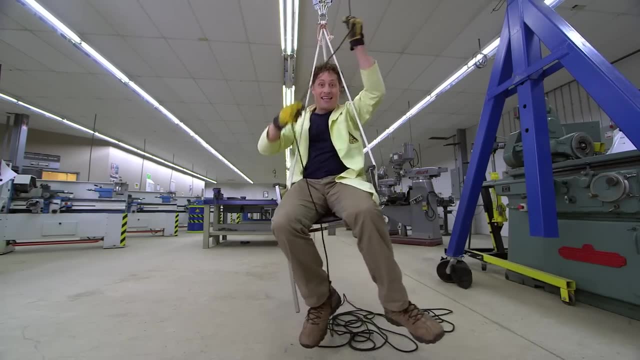 with the power of pulleys and I don't need to use two hands. In fact, I only need to use one finger to hold myself up and my thumb, obviously, to hold the rope. That is the power of pulleys. 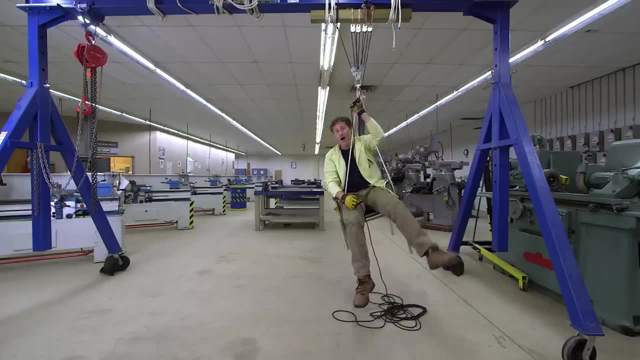 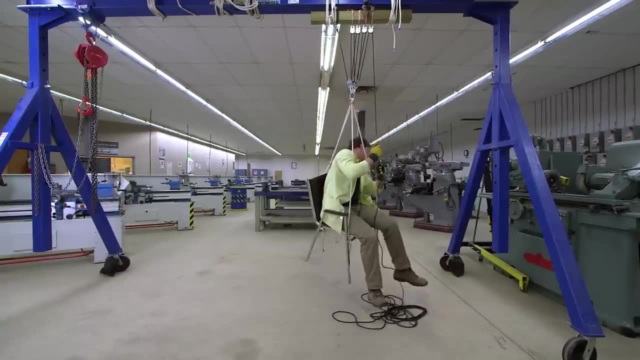 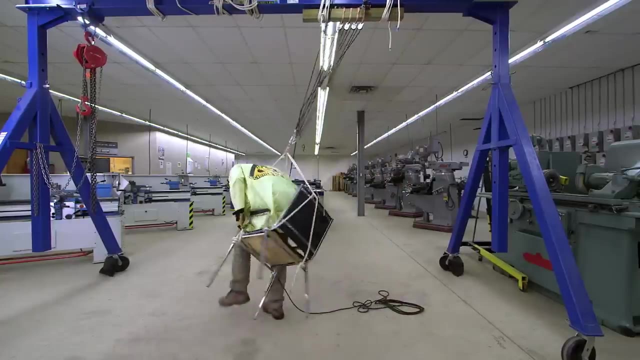 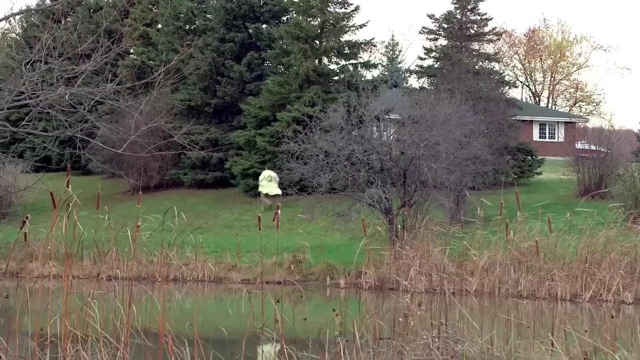 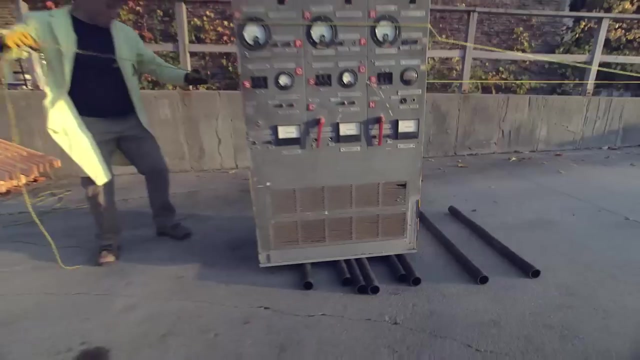 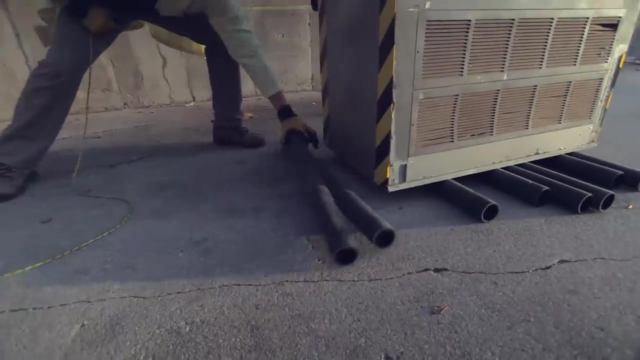 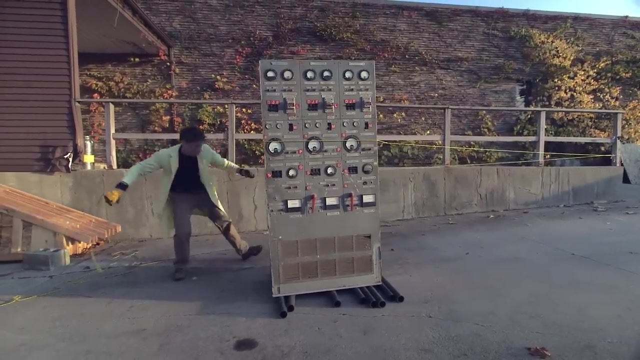 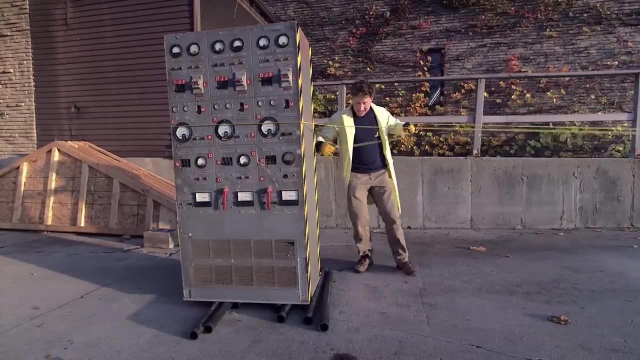 I can almost make myself fly. Well, almost. Now back to the particle impulse controller, Letting myself down. Particle impulse controller, Let's go Wait. All right, I've been able to use this pulley to lower it down the hill at the speed I want to go. 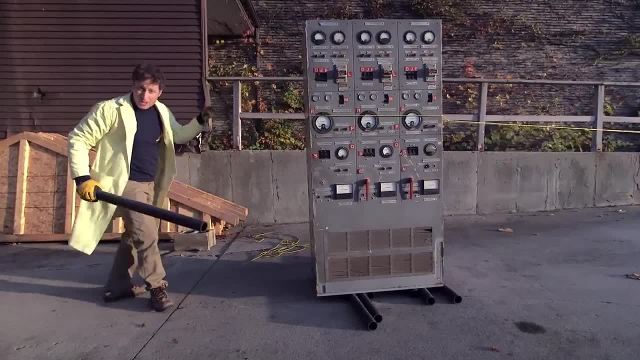 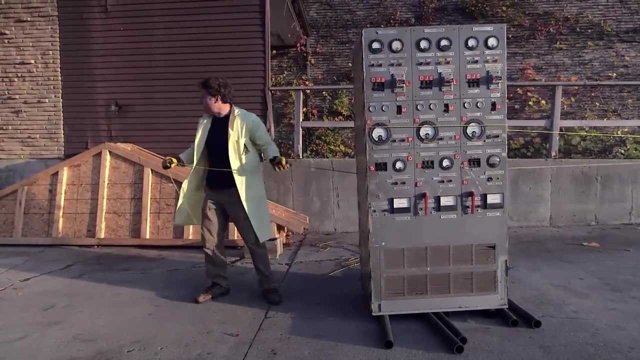 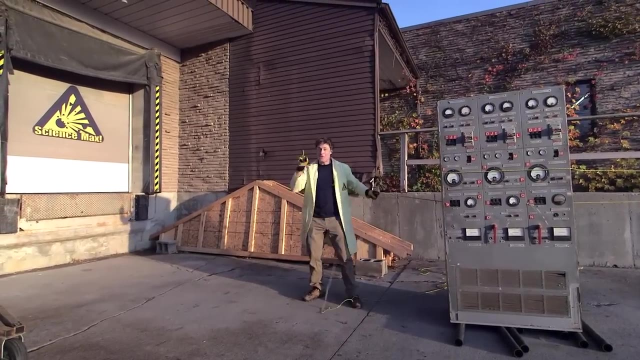 Interestingly, I'm using the pulley, not to make it lighter, but to just change the direction of force, And I managed to get it right here at the bottom. Now I've got to get it up onto the loading dock, so I think this is where I need a ramp. 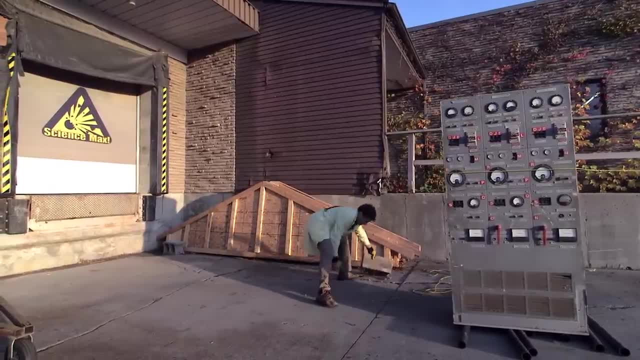 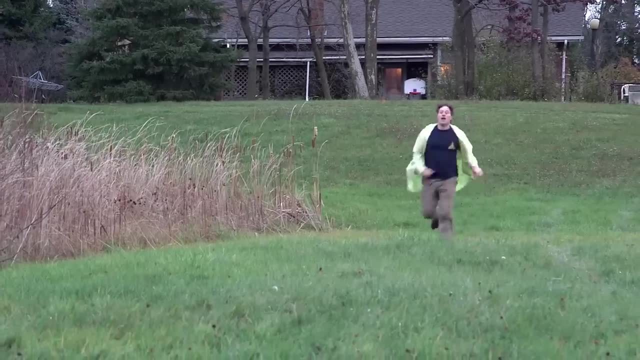 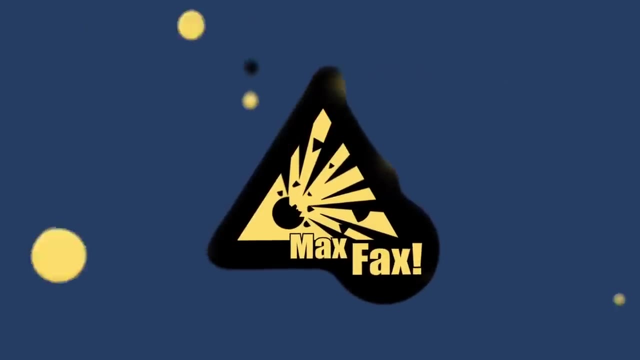 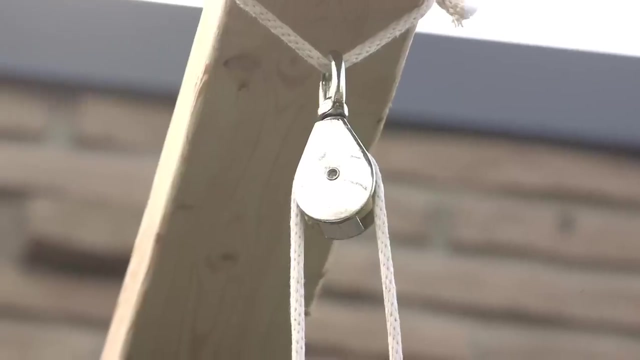 Whoa, Whoa. Oh, Here is something mind-bending you can do with pulleys. These buckets are attached to the table through a pulley. There's nothing holding this table up, except for the weight of the buckets pushing down on the table. 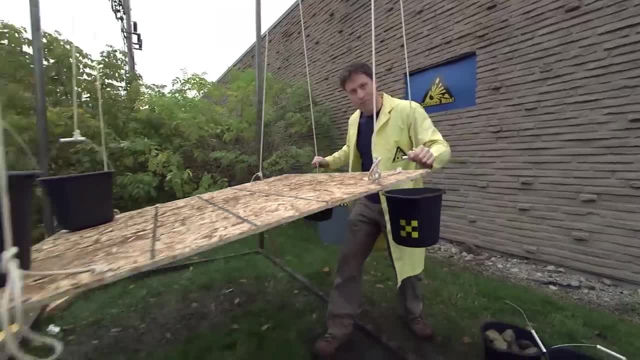 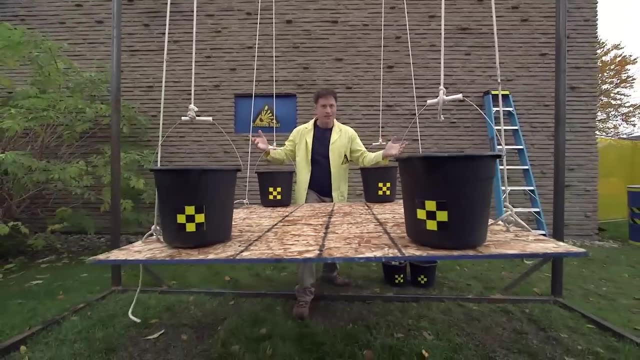 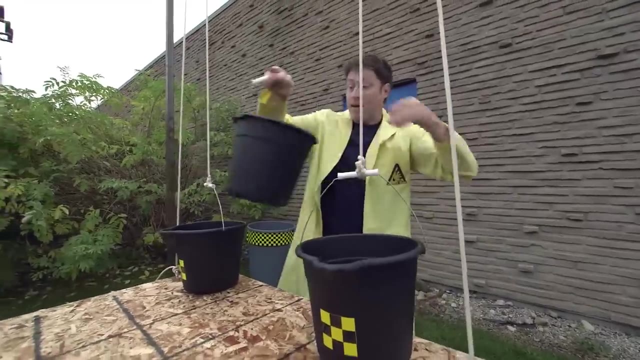 So if I took the buckets off the table, the weight of the buckets pulls the table up, But because the buckets are on the table, everything is in balance. Mind-bending right. Okay, wait, It gets better. If I took a weight and I put it on the table, the weight of the buckets isn't enough to keep the table up. 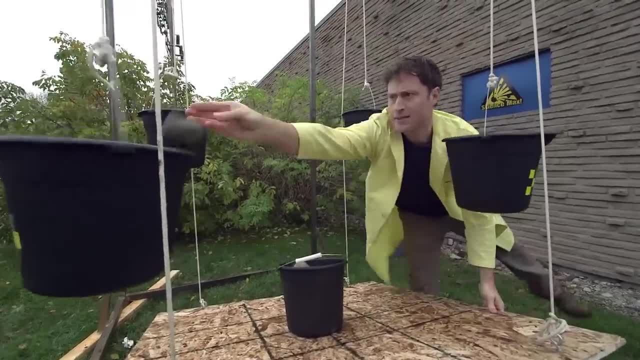 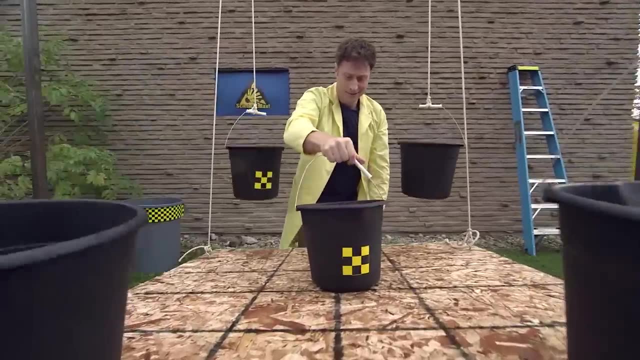 So I have to add more weight to the buckets, So the buckets pull the table. So I have to add more weight to the buckets to keep the table up. And there you have it. It's weird, It's mind-bending. 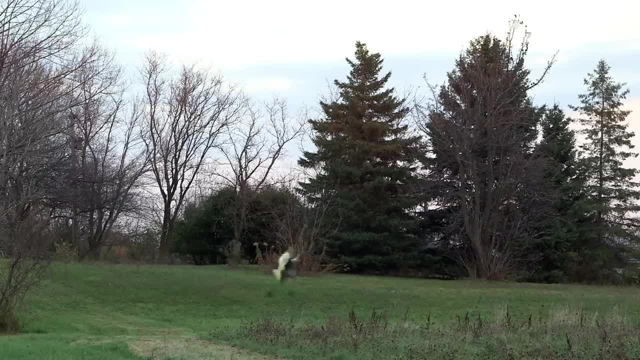 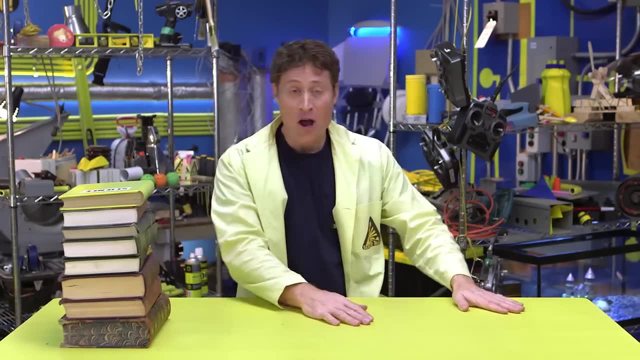 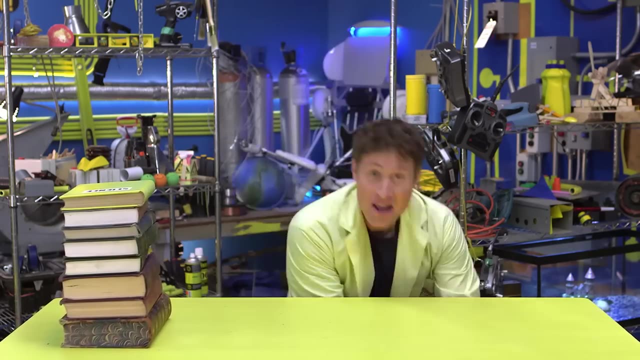 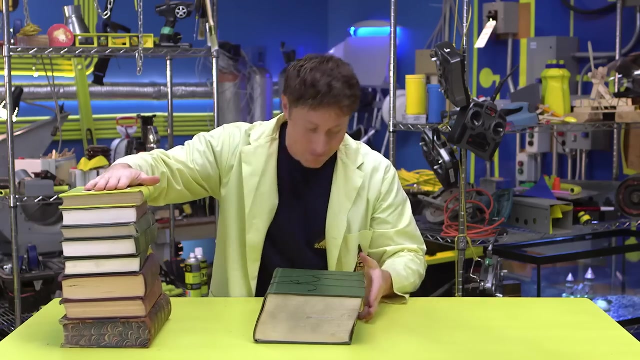 It's science. It's science, Okay, Okay, Ramps. Ramps are a great way to move something up. I will demonstrate using- you guessed it- a book. Let's say I wanted to move this heavy book on top of this stack of books using just this little string. 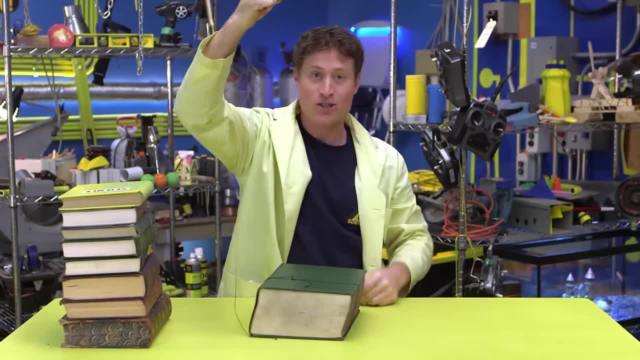 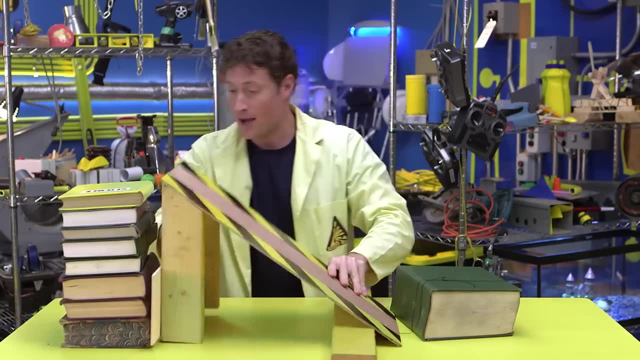 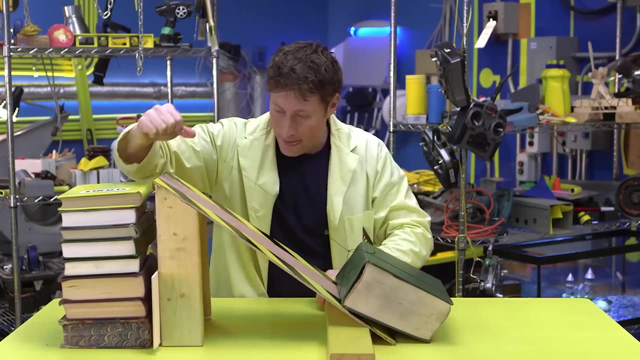 Watch what happens: The string breaks. But if I built a ramp to get the book on top of this stack and I use the same kind of string, watch what happens. this time, You see, the ramp destroys the book. It distributes the force. 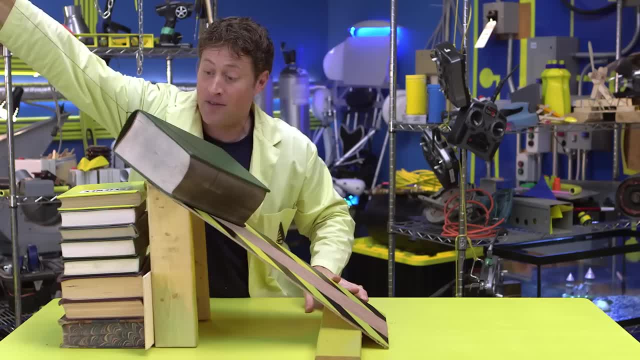 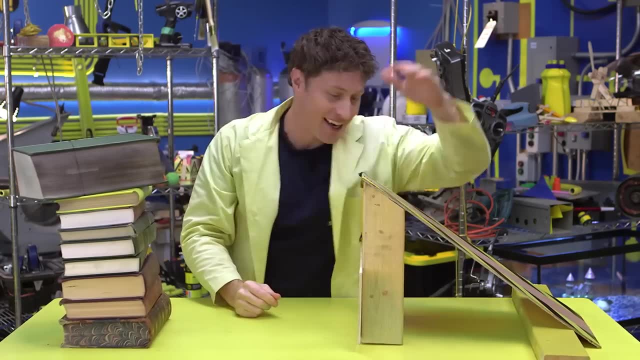 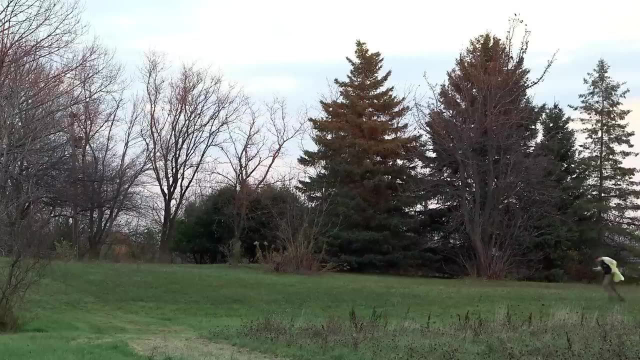 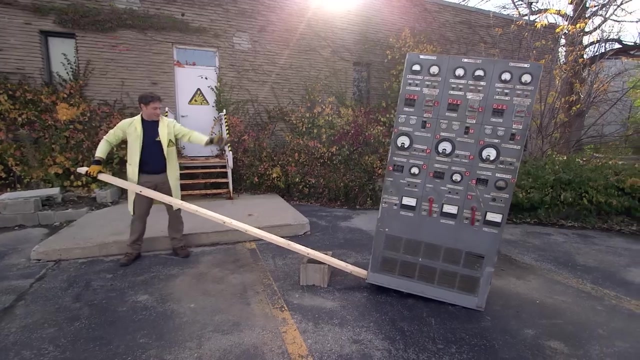 So you use less force to pull the book over the same amount of distance and I can get it up to the top of the stack of books and the string doesn't break. So, ramps, Let's put them into action. My simple machines have worked great. 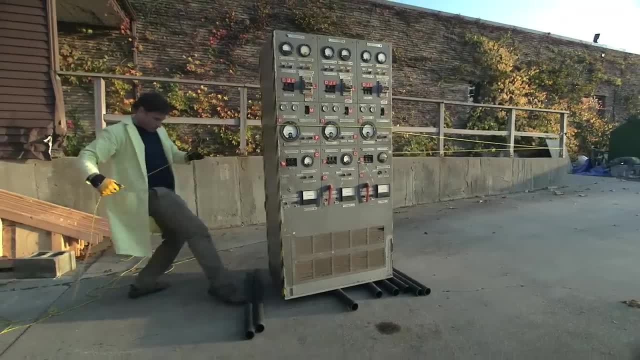 I've managed to get the particle impulse controller all the way to the top. I've managed to get the particle impulse controller all the way to the top. I've managed to get the particle impulse controller all the way to the top. I've managed to get the particle impulse controller all the way to the loading dock. 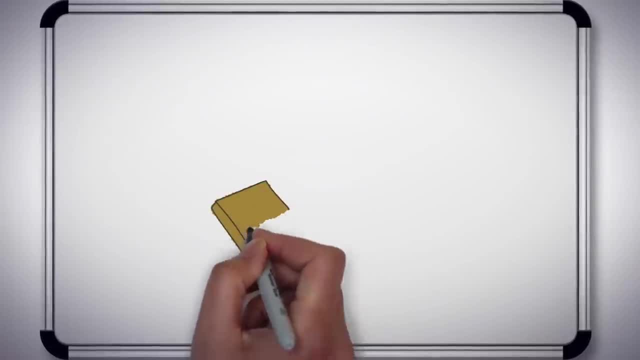 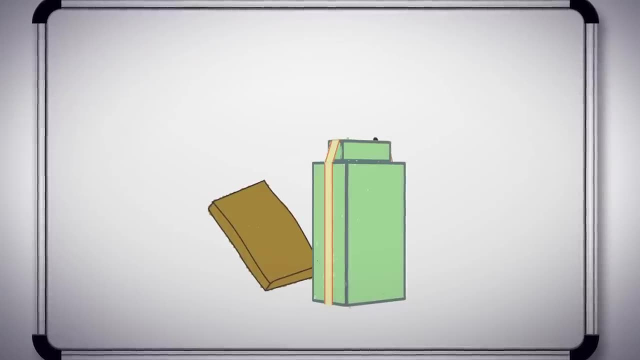 But now it's time for the hardest job. What I need to do is build a ramp that goes from the ground up to the loading dock. Then I need to pull the heavy impulse controller up the ramp. The best way to do that is to use a system of pulleys. 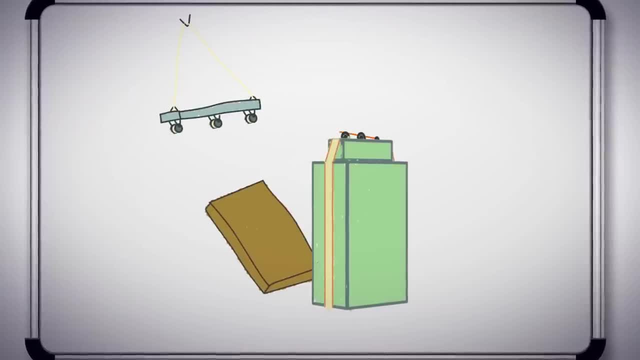 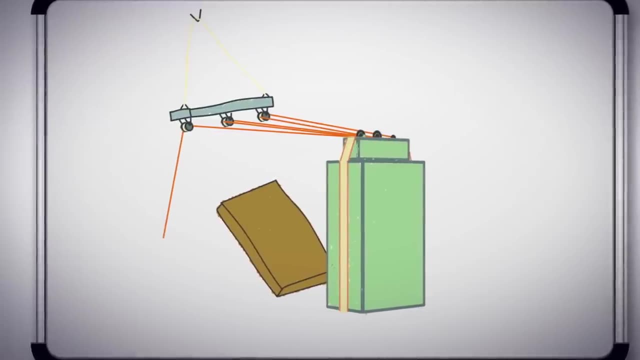 I have three pulleys on one end and two pulleys on the controller. Because I have five pulleys working together, I'll only have to lift one fifth of the weight. The plan is to get it tipped over onto the ramp, then use rollers to help it roll up up to the top of the ramp. 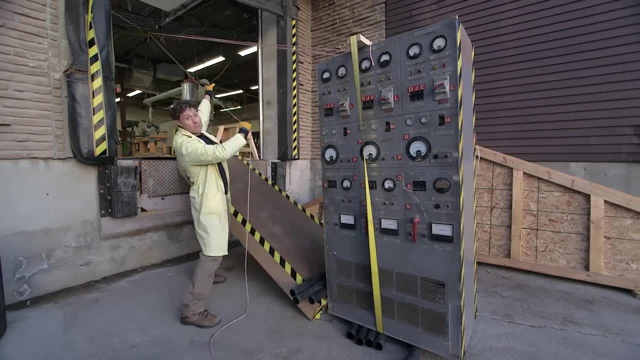 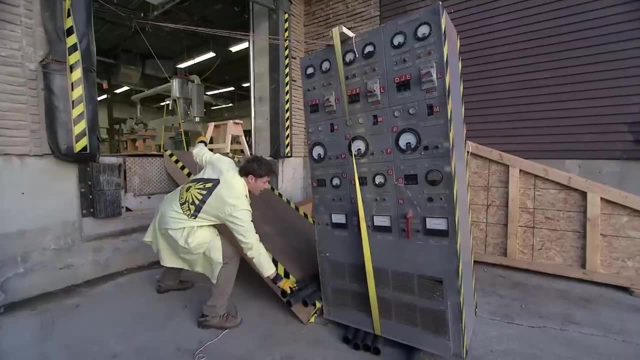 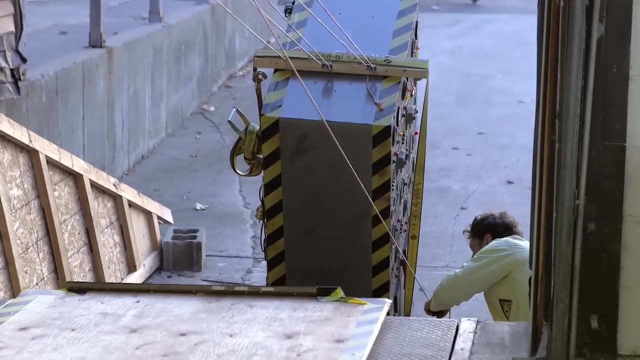 up as I pull on the rope. There's three pulleys on that piece of wood over there And I got two pulleys on this piece of wood here And now if I pull and I carefully put the rollers underneath. careful, careful, perfect.